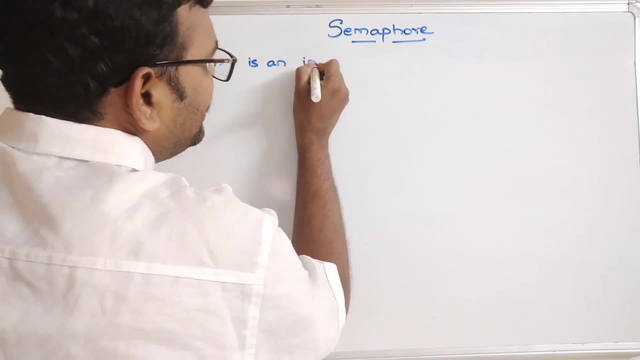 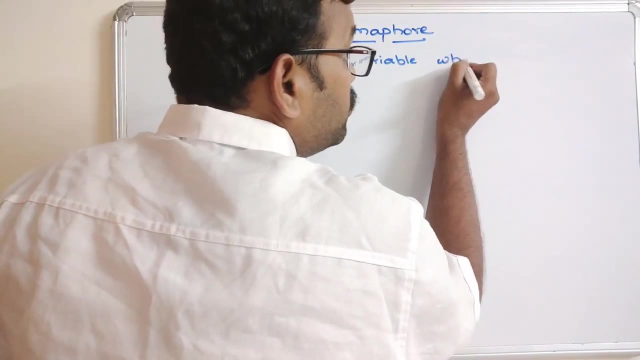 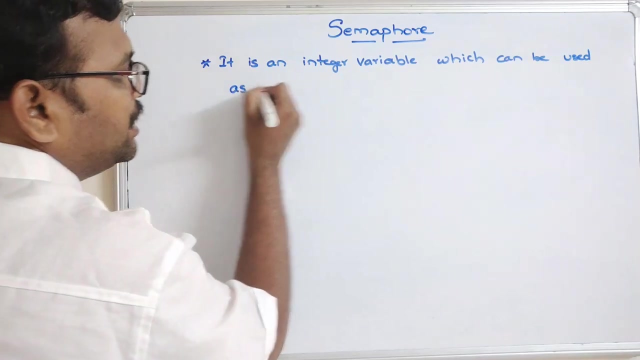 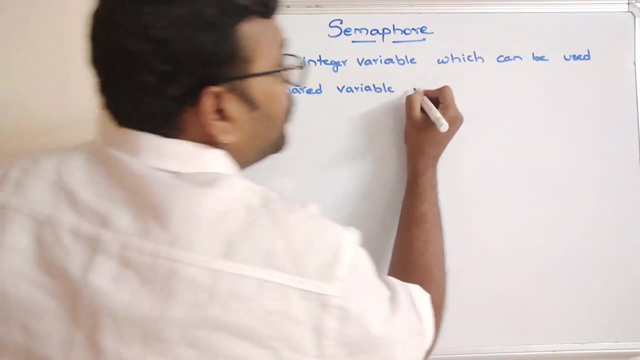 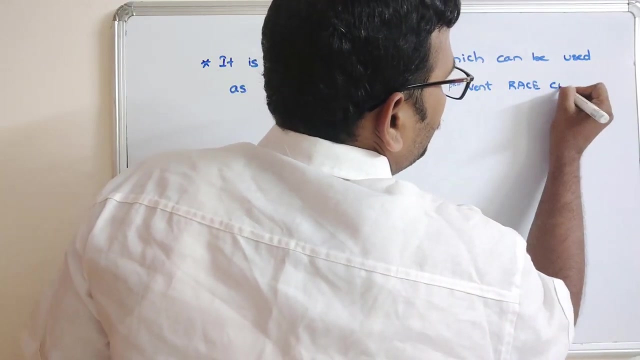 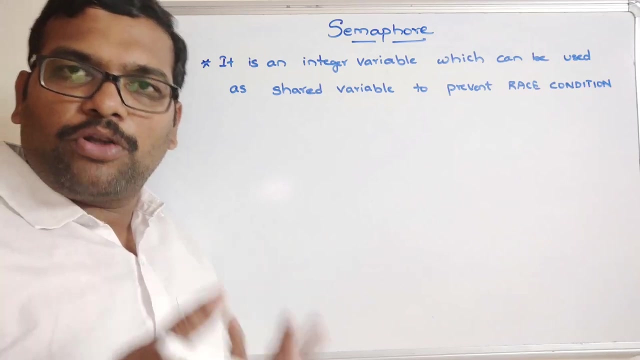 semaphore is an integer variable which can be used as a shared variable, So which can be used as a shared variable To prevent waste condition. So actually in our previous session we have discussed about the thread concept, a process concept, and we have seen the process synchronization right. 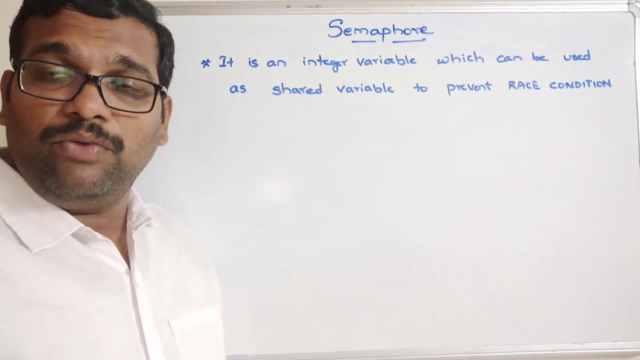 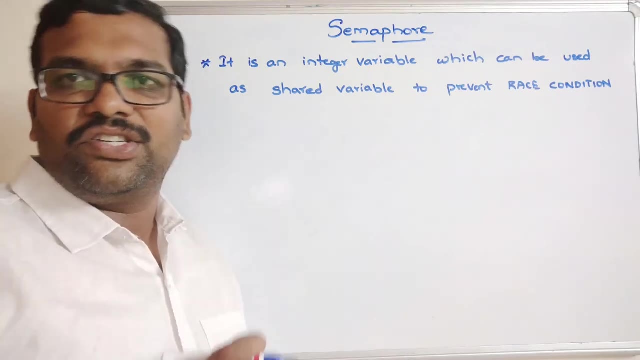 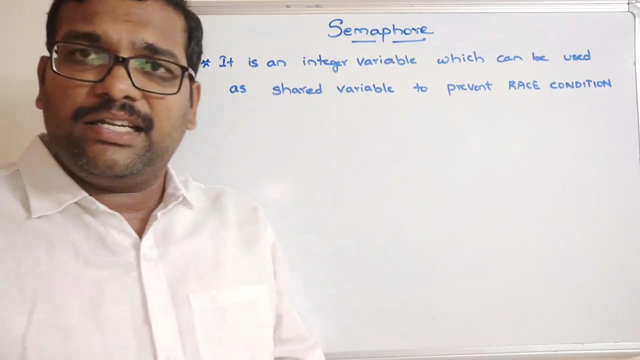 So there we have seen the critical section problem. So only one process should be entered into the critical section so that other process need to wait for its execution until the critical section is available. right, so that we have seen in our previous session and that in order to solve the critical section, 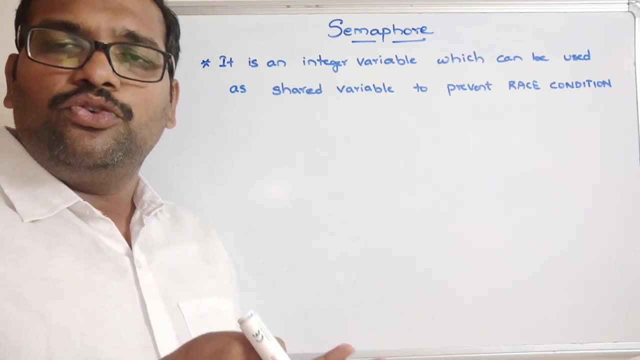 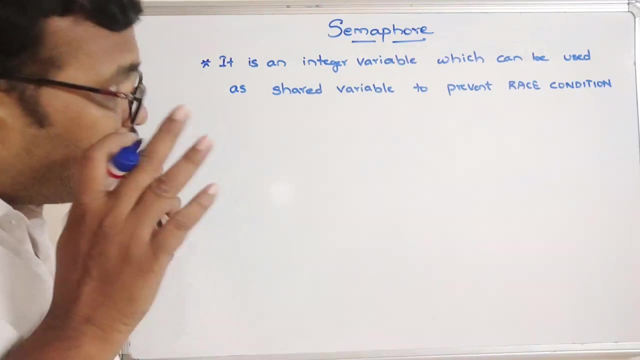 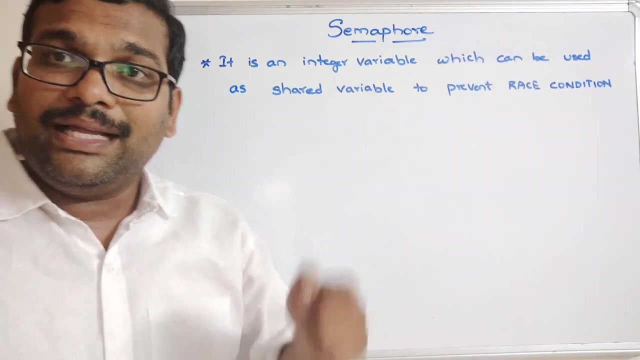 so the three conditions should be satisfied. that one is a mutual exclusion. so mutual exclusion means at a time only one process should complete its execution right. so for that purpose we will use a semaphore as a solution to prevent the race condition. so race condition means if two. 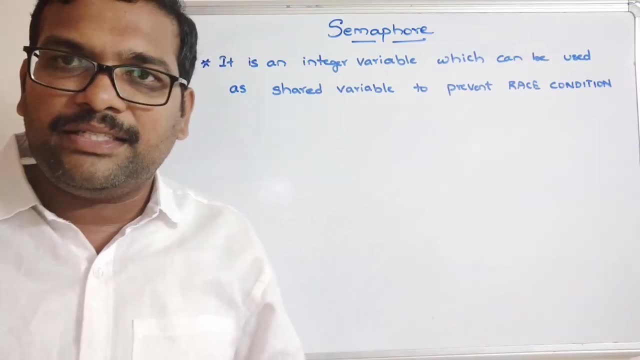 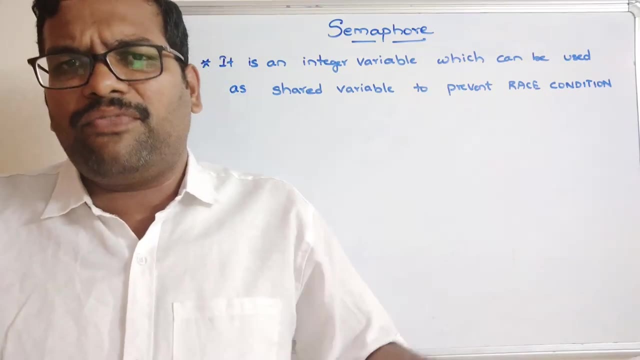 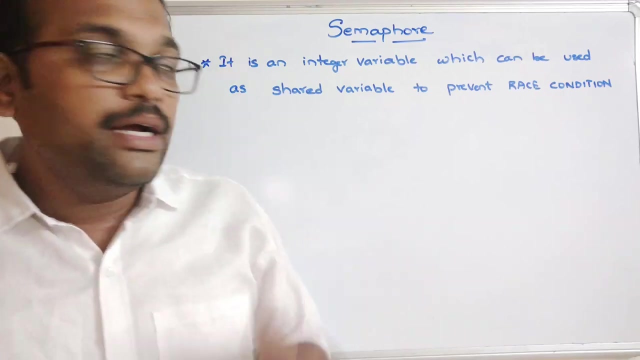 processes are executing concurrently, there might be a chance of getting the inconsistency on data so that we call it as a race condition. both the process will be having a different results and both the process will be treating that their own result will be the correct one, right? so such 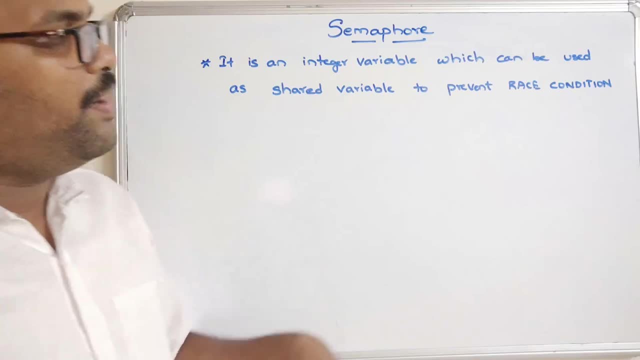 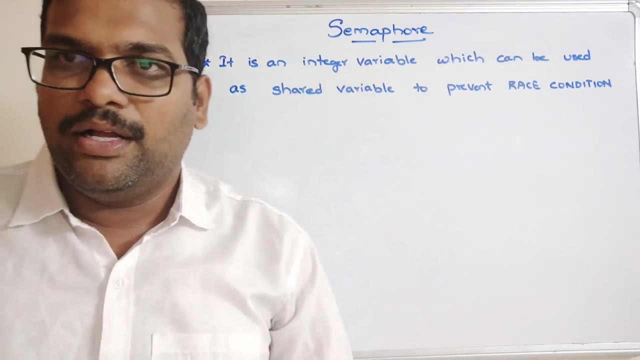 type of thing we call it as a race condition. so, in order to prevent that race condition, we will use a semaphore as a integer variable which can be used as a shared variable. so, actually, if we are using the process synchronization, if we are using some multiple process which are being 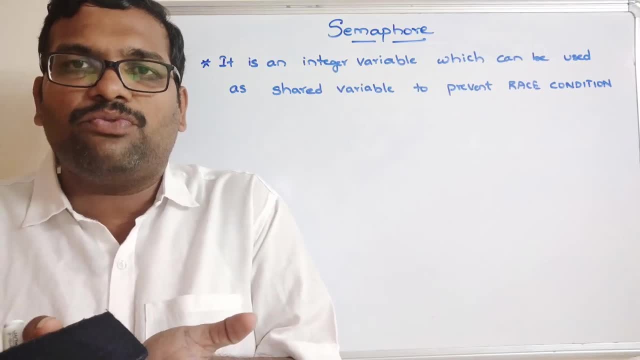 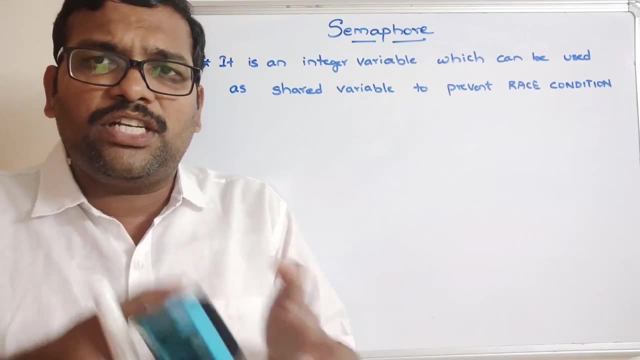 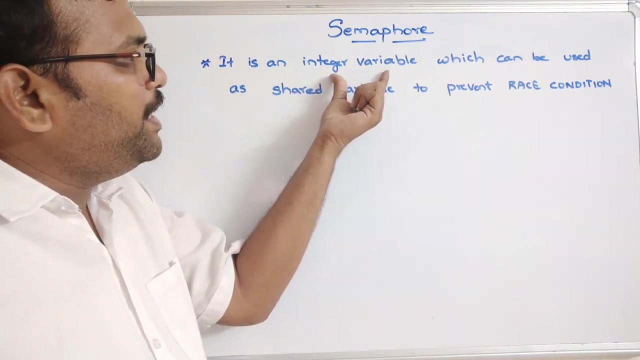 executed continuously, some shared resources will be. i mean, some sort of resources will be shared between both the process. right so those resources may be the variables or functions or any other resources. right so this integer variable will be acting as a shared variable among the different processes in order to prevent the race. 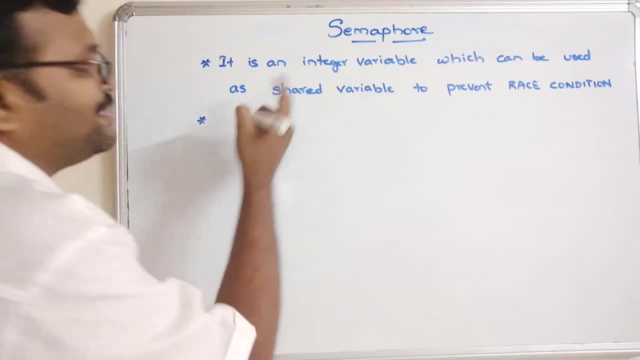 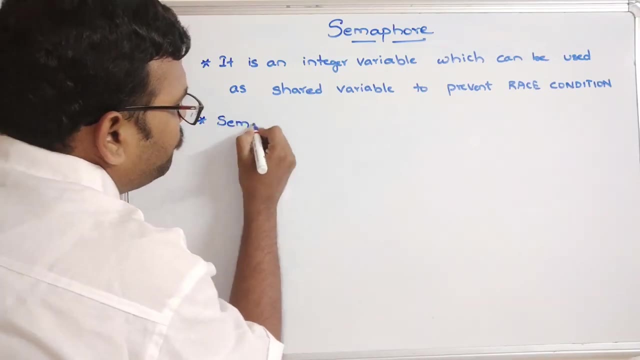 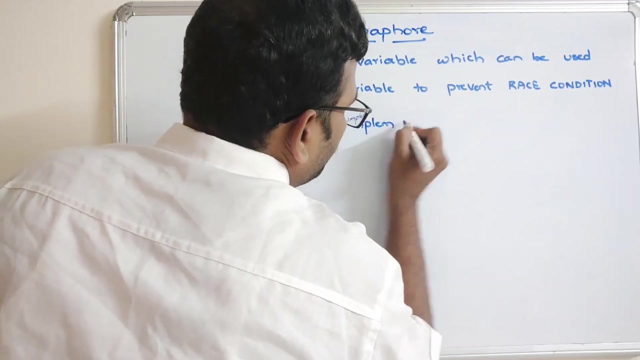 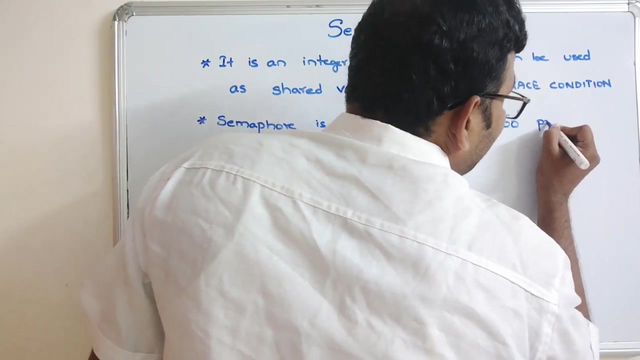 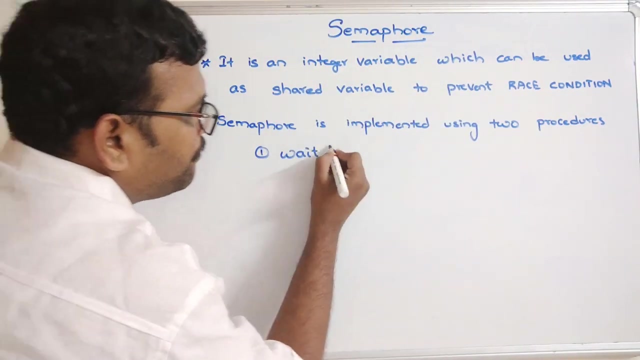 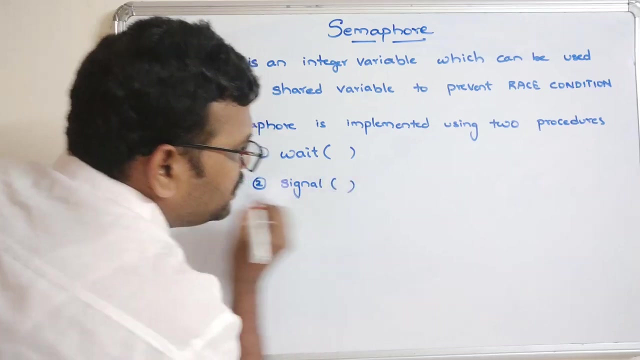 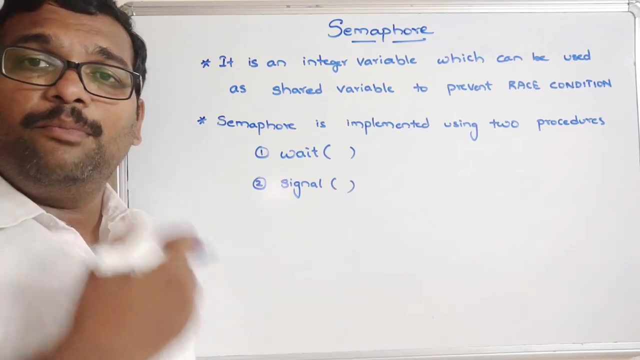 condition. and see here, this semaphore is implemented with the help of two procedures. so see, semaphore is implemented, implemented using two procedures, two procedures. so first one is a wait procedure and the second one is a signal procedure. signal procedure: so this will tell the process whether it is able to enter into the critical section or 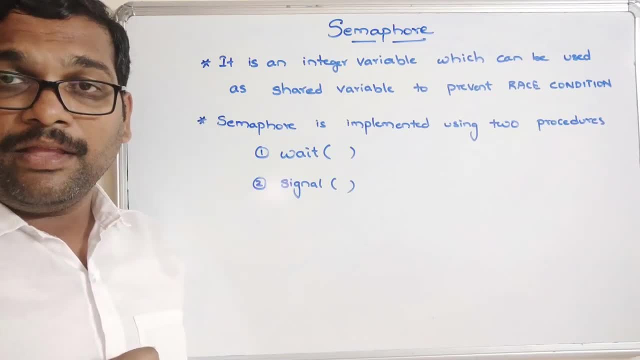 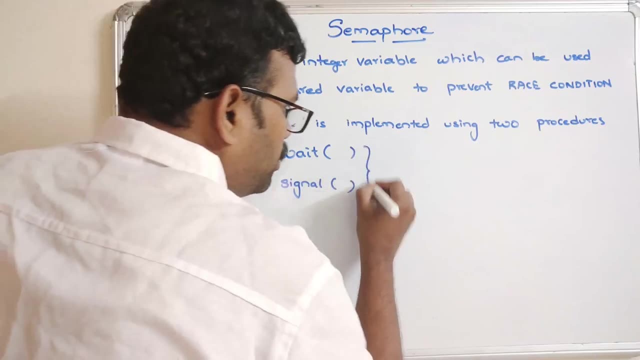 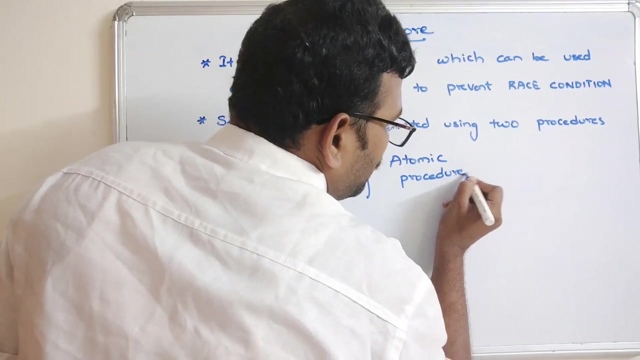 it has to wait for some time. so for that purpose we are going to use this wait and signal in order to implement the semaphore and see both or atomic procedures, both are atomic procedures. so here the term atomic procedures means until it completes its execution. it should not be. 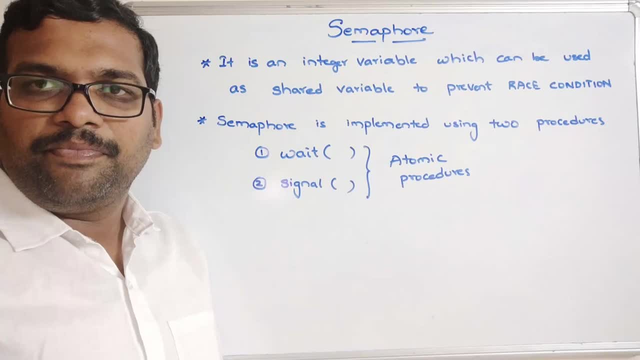 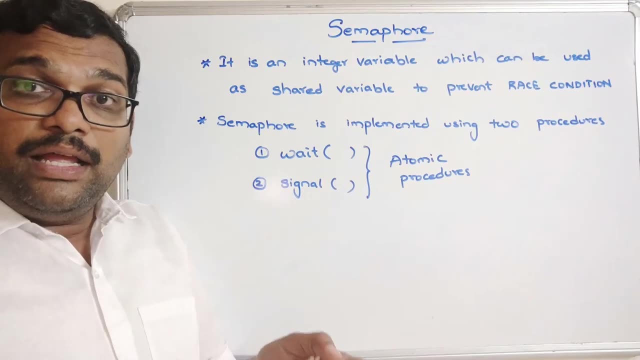 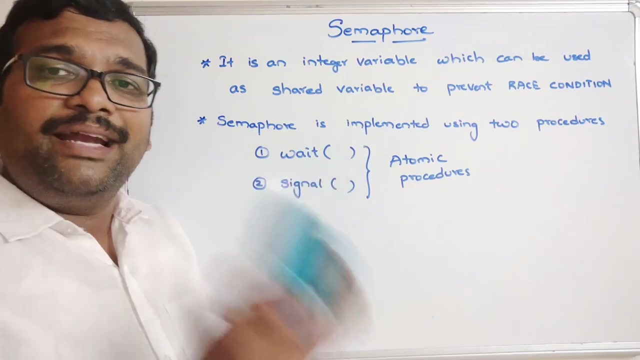 interrupted by any other process, right? so if the wait process, if the wait procedures being executed by the process, so the until it completes its execution, the until the process completes its weight procedure, no other process should interrupt this one. so, after successful completion of all the instructions available in the weight, 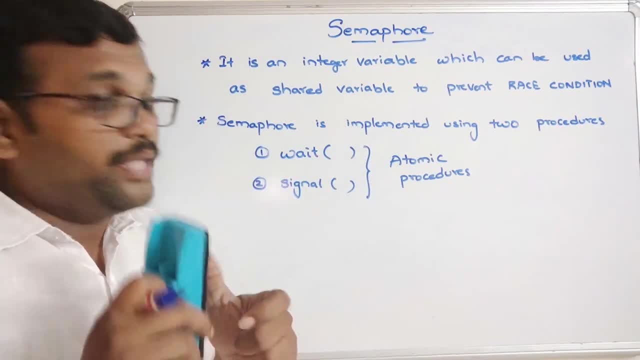 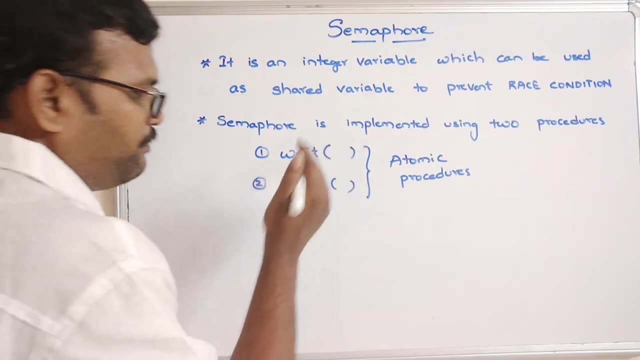 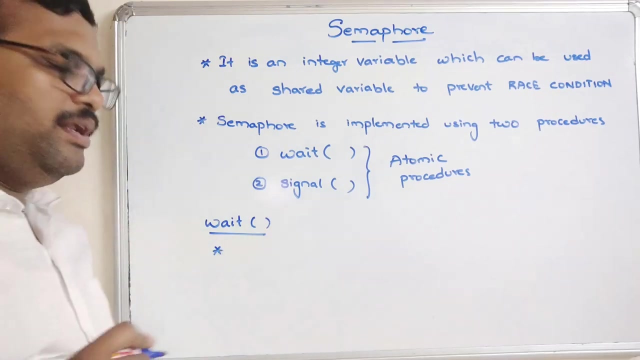 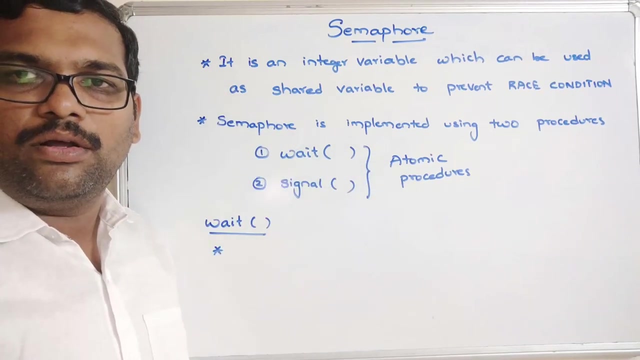 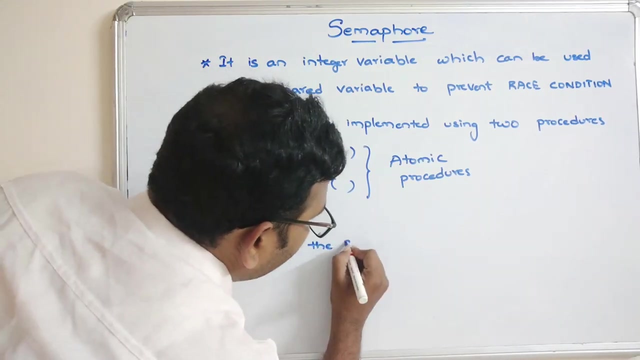 then only the next process will be being executed. so that's why we call it as an atomic procedures, so no process will interrupt, right. so let us take the weight procedure, weight procedure. so in this weight procedure it mainly tell that whether the process is able to use the critical section or not, so it gives the status for the process. 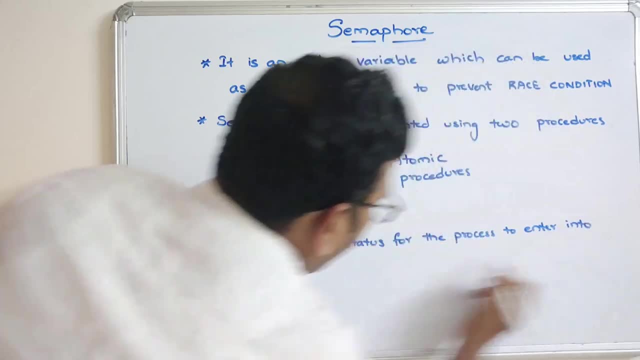 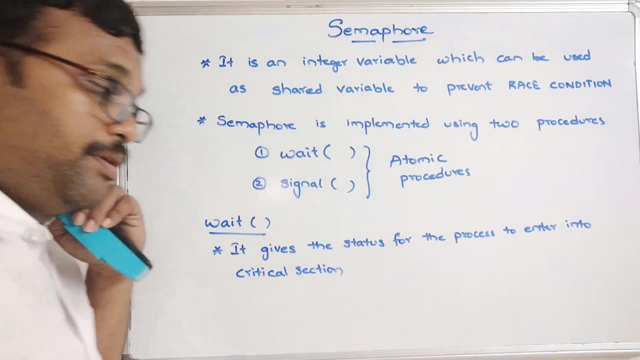 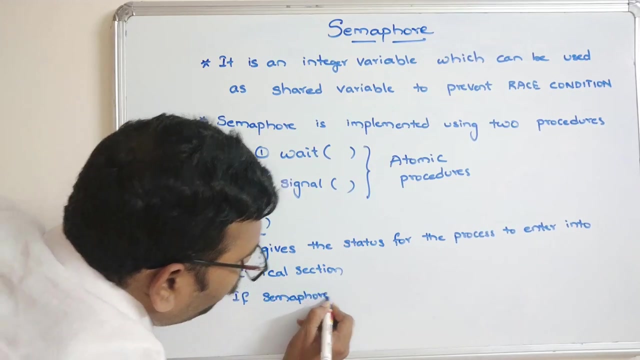 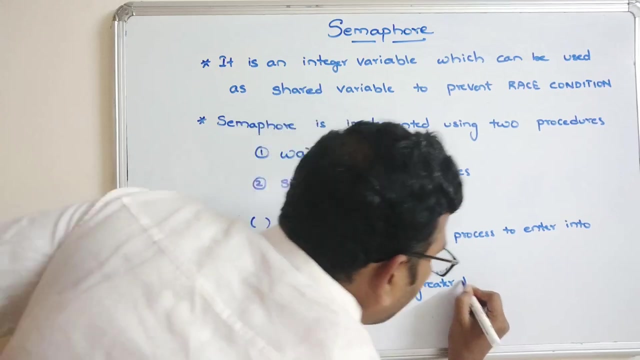 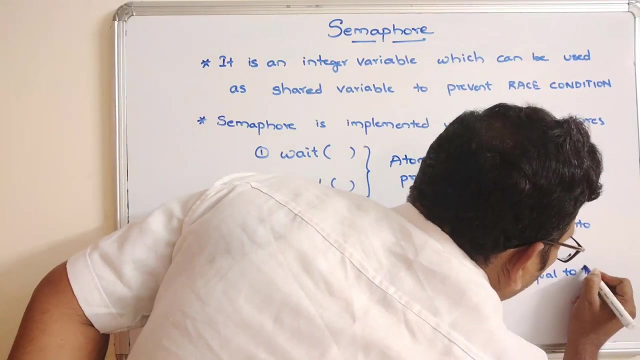 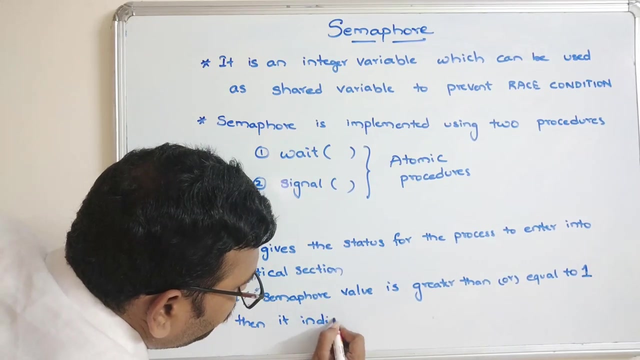 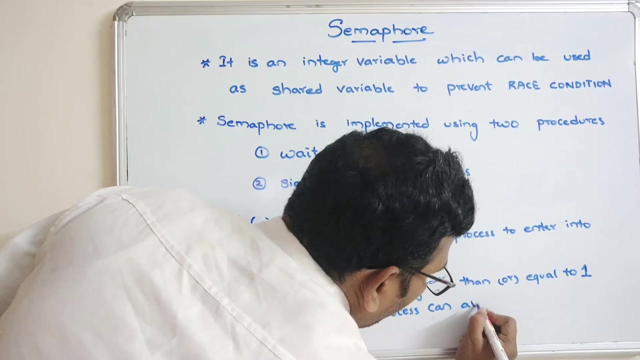 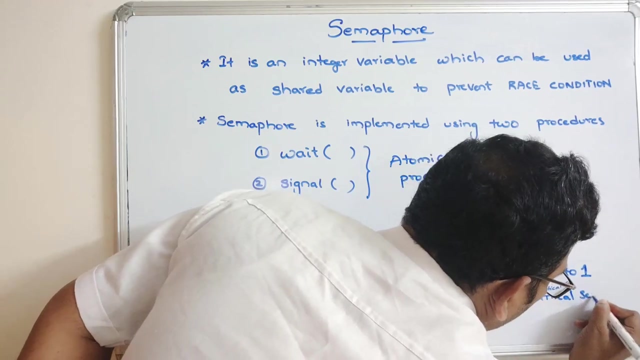 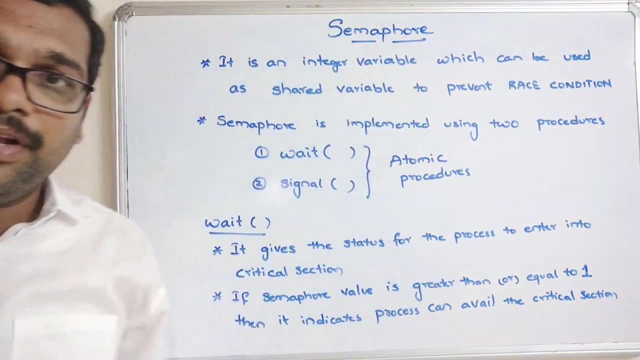 to enter into critical section. critical section right. and if the semaphore value, if the semaphore value is greater than or equal to one one, then it indicates. it indicates process can avoid the critical section. so the process can enter into the critical section. that means so, as we said, that the semaphore is an integer variable right, so integer variable. 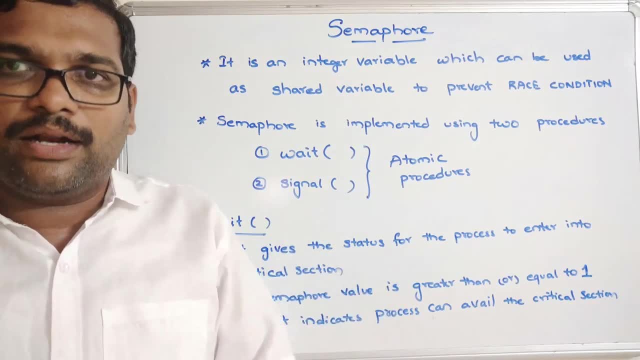 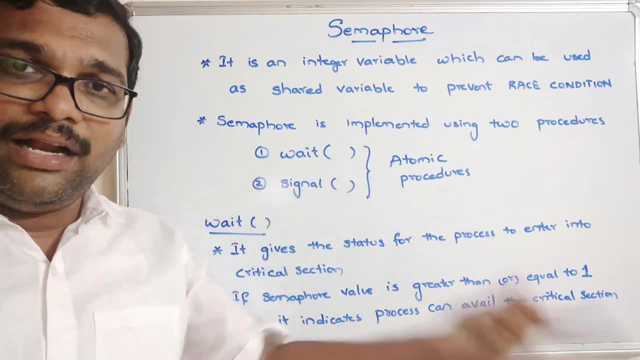 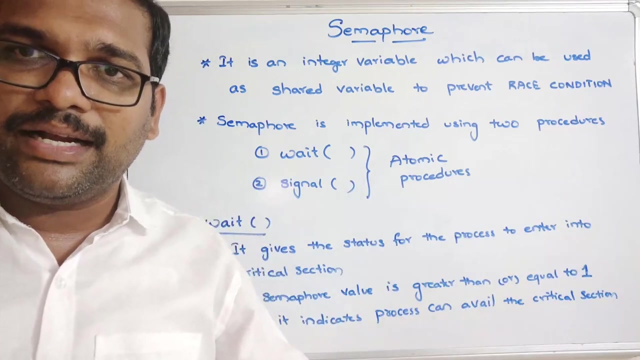 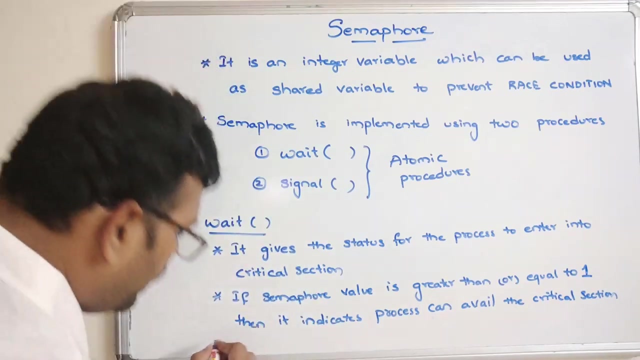 if that integer variable is a greater than or equal to one, that implies the critical section is available for the process. so a process can enter into the critical section, a process can enter into the critical section. so whenever the process enters into the critical section, the semaphore value will be decremented. the semaphore value will be decremented. so 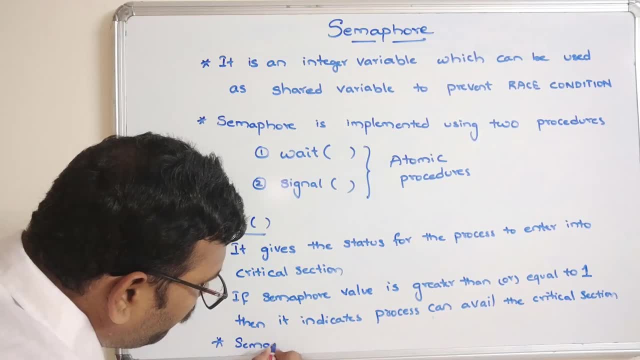 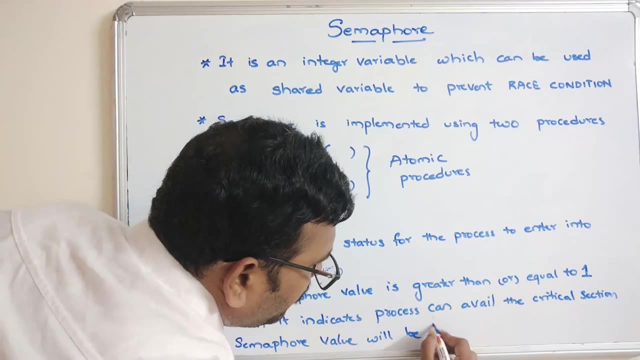 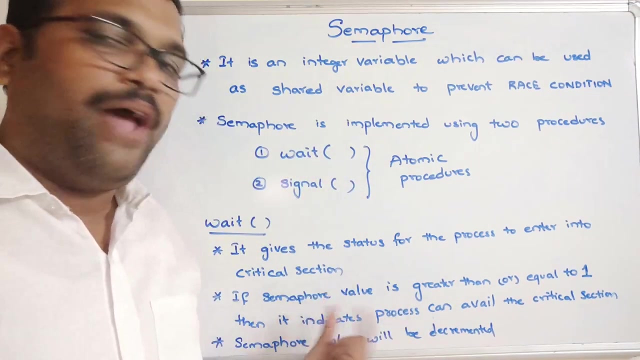 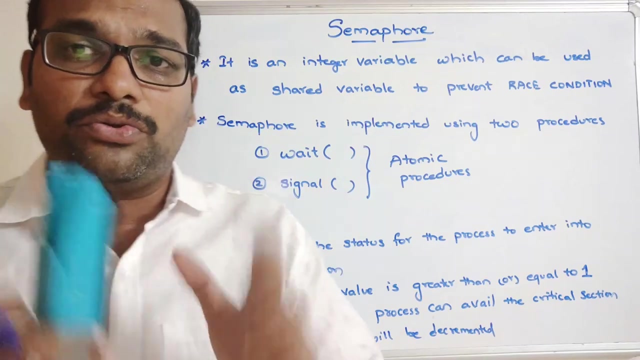 immediately what happens. so semaphore value, semaphore value will be decremented. so just for understanding, uh, let us assume that semaphore value is nothing but the number of resources. okay, so just for understanding, semaphore value is a number of resources. so if there are any resources available, that means if there are, if the 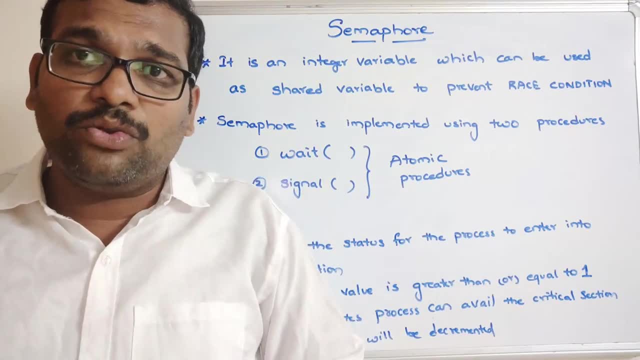 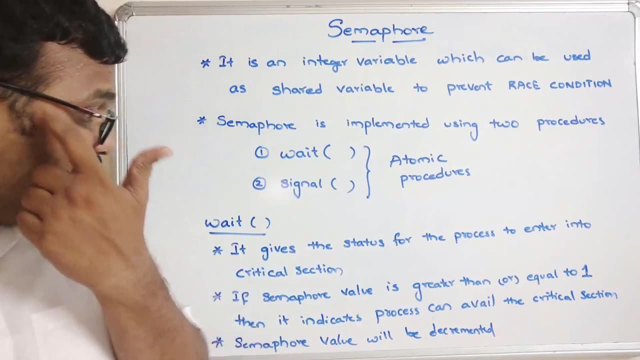 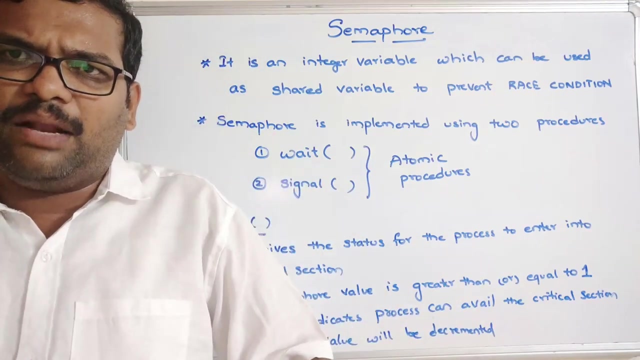 semaphore value is one that in that implies one resource is available, so automatically the process can utilize that particular resource right. So in such a way, if the semaphore value is greater than or equal to 1, that implies some sort of resources are available and that can. 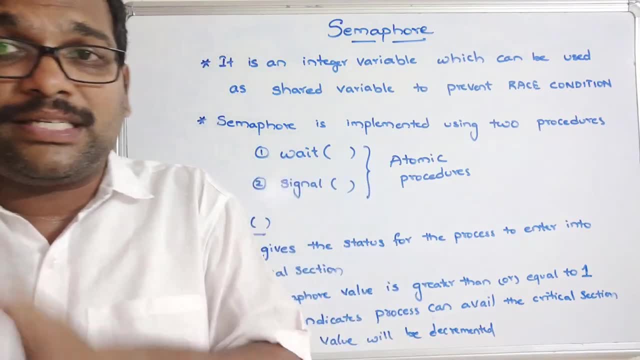 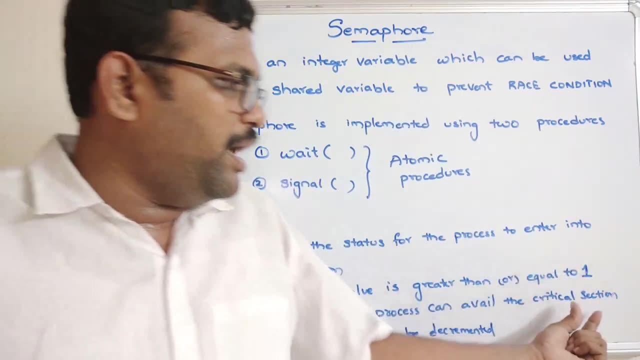 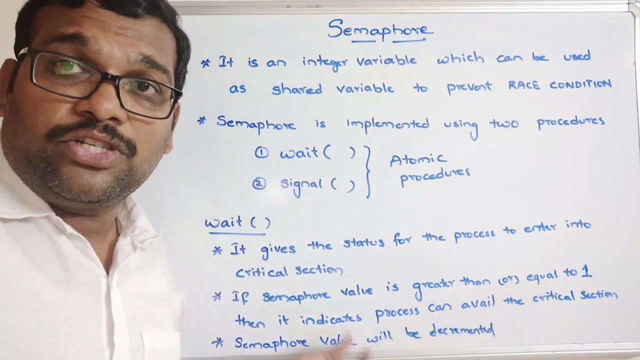 be utilized by some other process. So a process can avail the resources which are available by entering into the critical section Immediately. after entering into the critical section, immediately the semaphore value should be decremented. So if the semaphore value is not decremented, that implies there are still the resources available. right, It indicates: 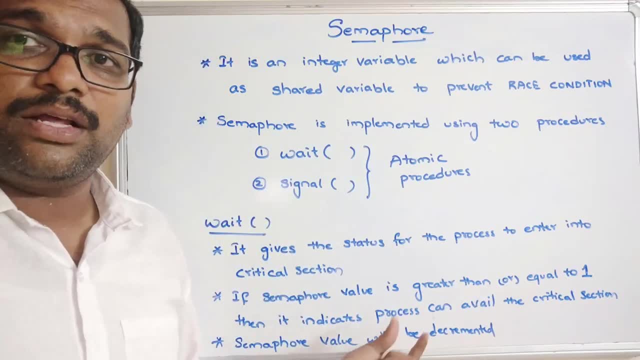 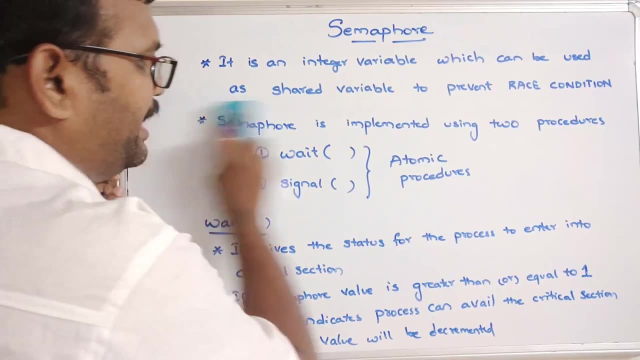 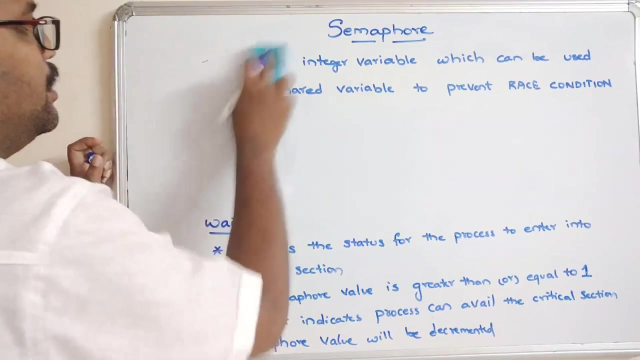 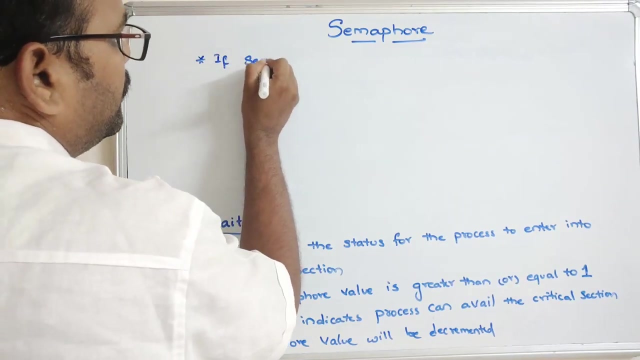 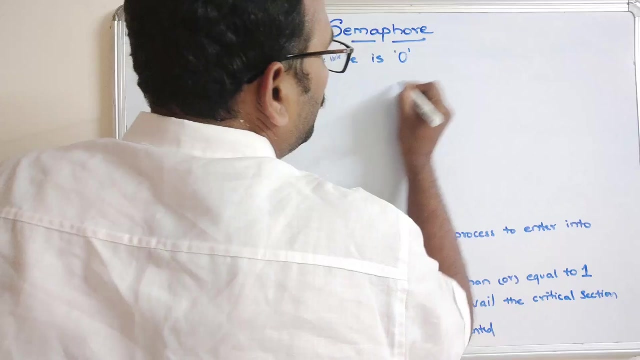 that still, the resource is available, but the resource is allocated to the process, So we have to decrement the value, right? So the thing. and the next point: if it is zero, So if the semaphore value is zero, if the semaphore value is zero, then it indicates: 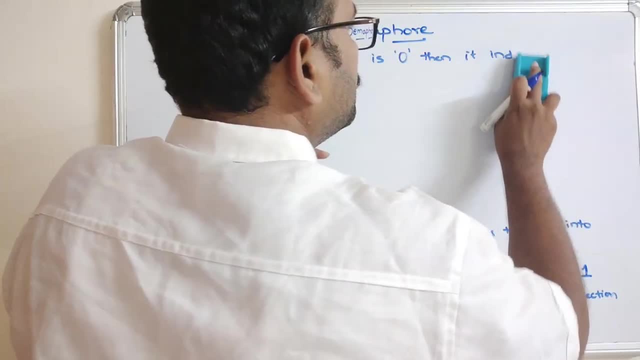 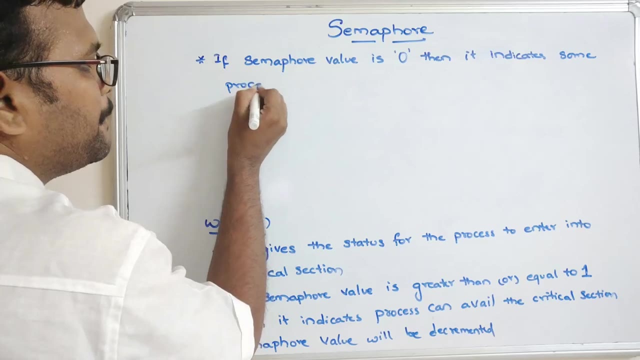 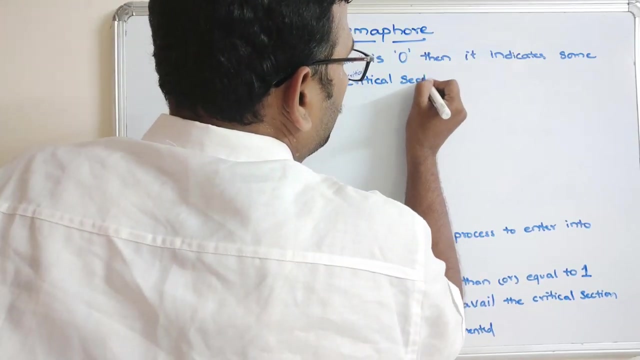 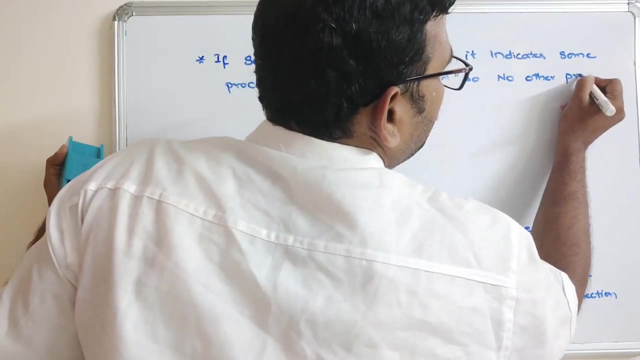 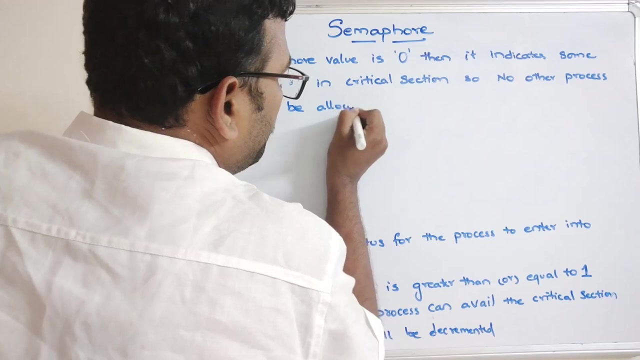 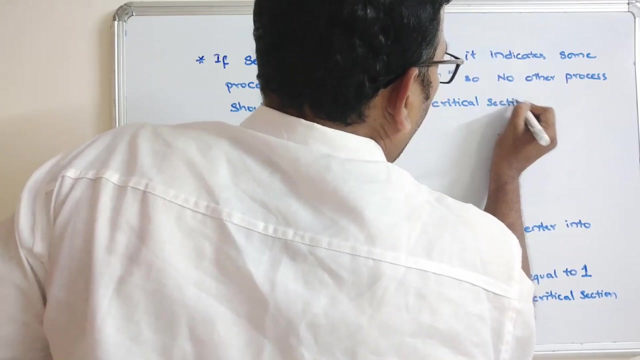 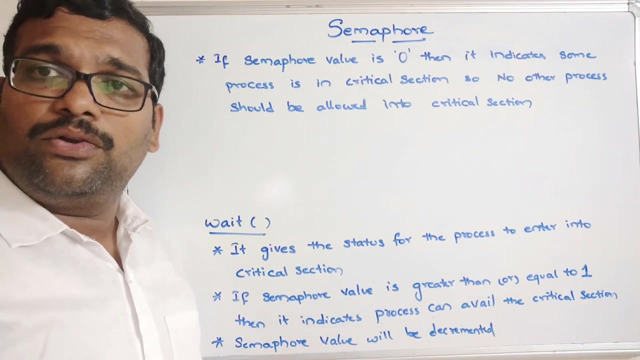 it indicates some process is in critical section, critical section, So no other process should be allowed. no other process should be allowed into critical section, right? So if the semaphore value is zero, that implies so just for now we have seen- the semaphore value is equal to number of. 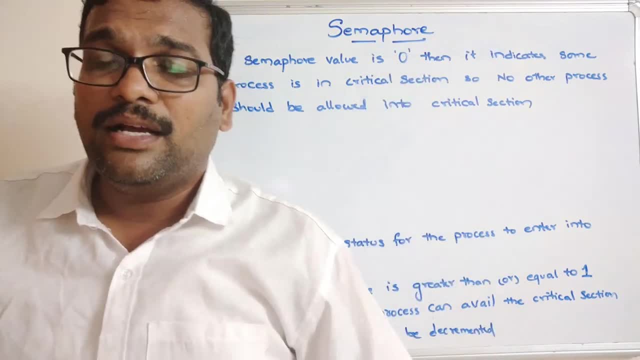 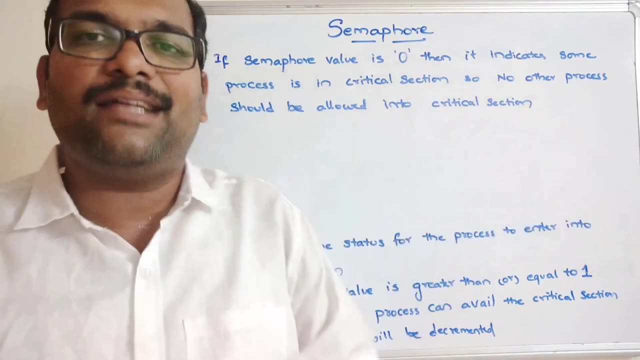 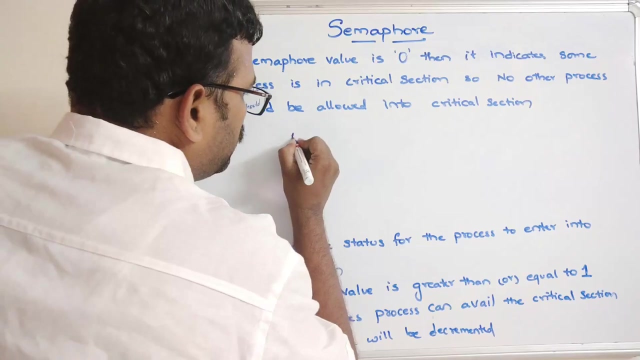 resources. if the number of resources are zero, that implies the all the resources have been availed by other processes. so the current process should wait until it gets the resources right. so if you write this same procedure with the code, so the code will be weight of semaphore. 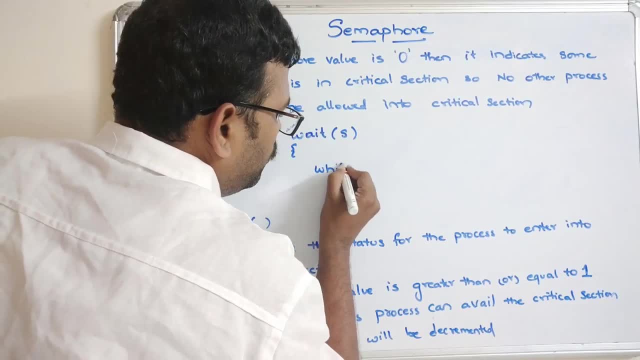 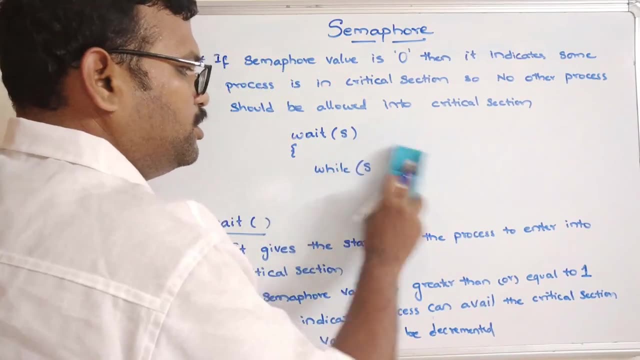 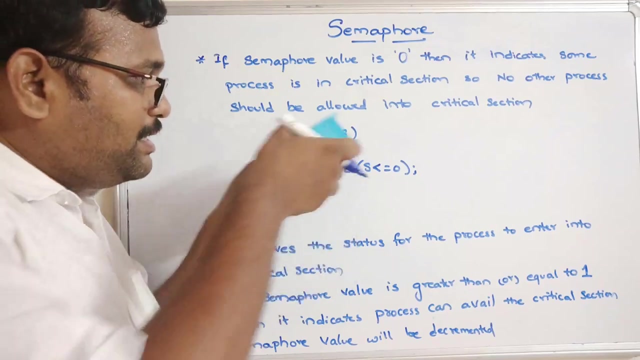 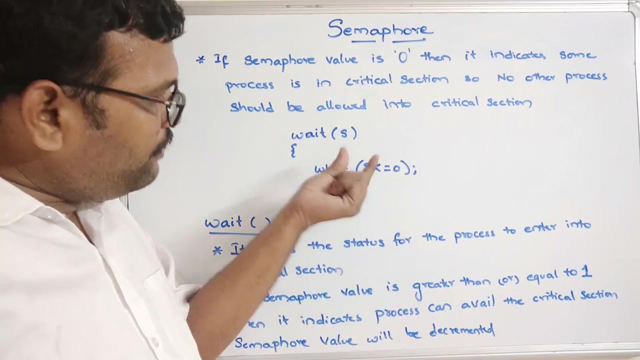 and write down the loop: while s less than or equal to zero. see while s less than or equal to zero semicolon. that means it will. it will be inside this particular loop until s is greater than one- i mean greater than zero, right? so if it is s is less than zero, it will wait in this particular 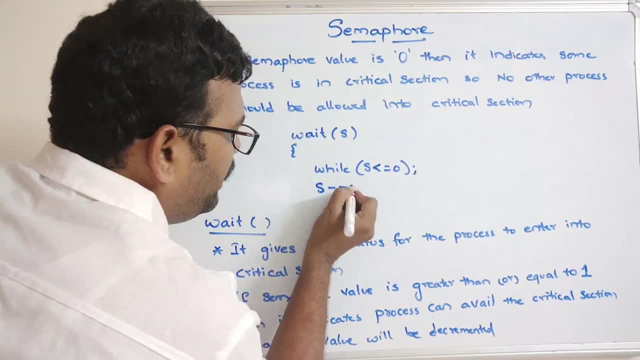 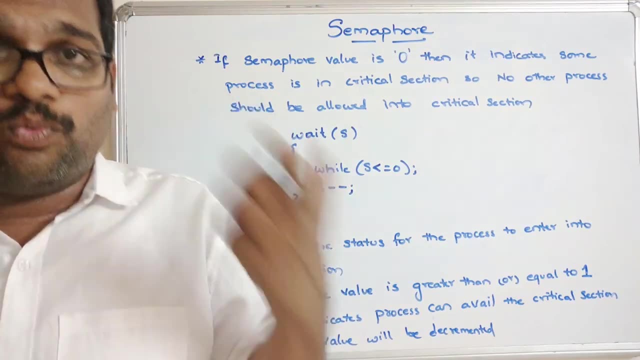 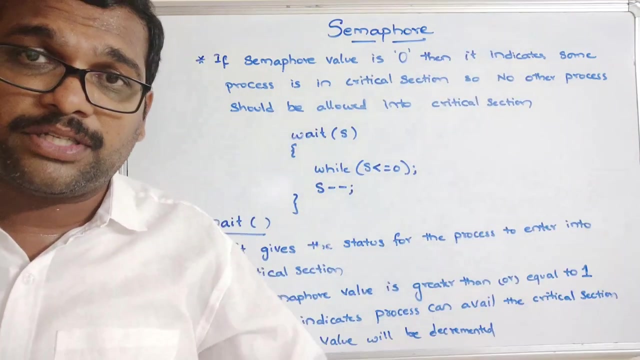 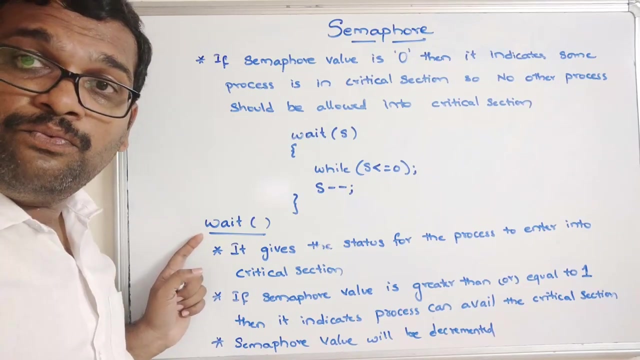 loop itself. immediately the s value will be decremented. the s value will be decremented, so that means if s is greater than zero, that means if s is equal to one, so automatically it will be decremented. it will be allocated by other process, allocated to other process, and that will be decremented, right? so this is the weight. this is a weight procedure. 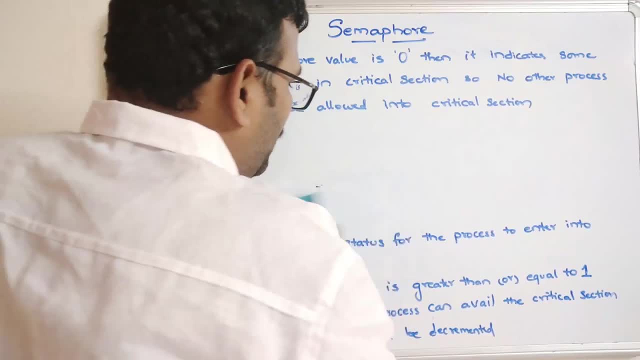 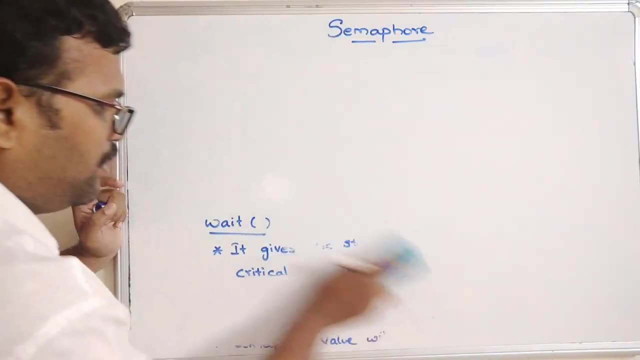 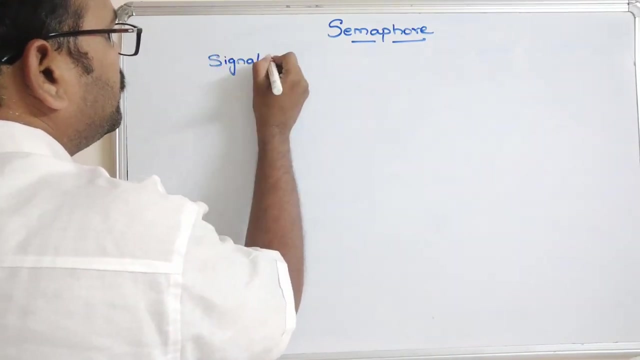 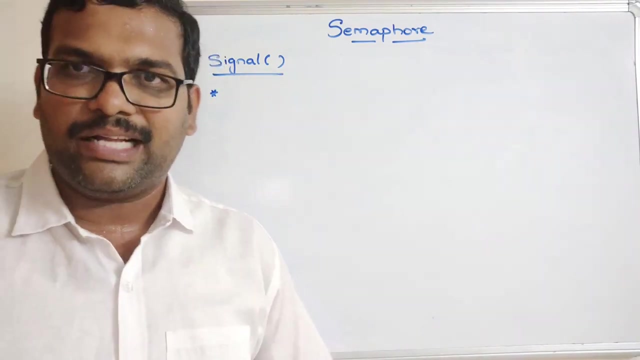 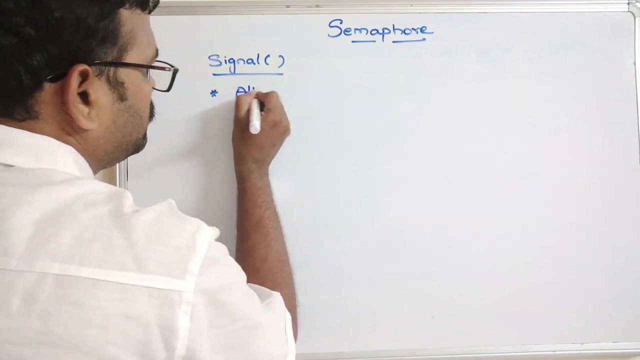 then signal. the second procedure is a signal procedure. second procedure is a signal procedure. so it's a very simple. so whenever the process completes its execution in the critical section, whenever it comes out of the critical section, immediately the semaphore value will be incremented right. so after completion of the process, 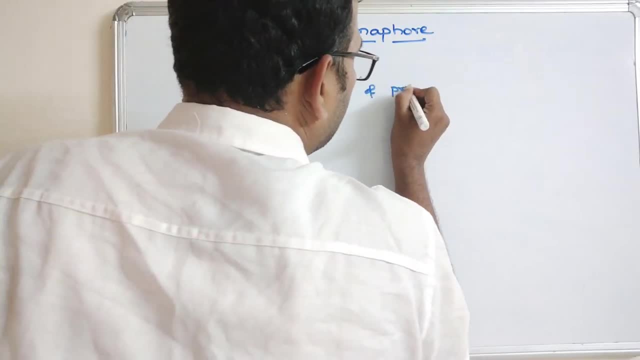 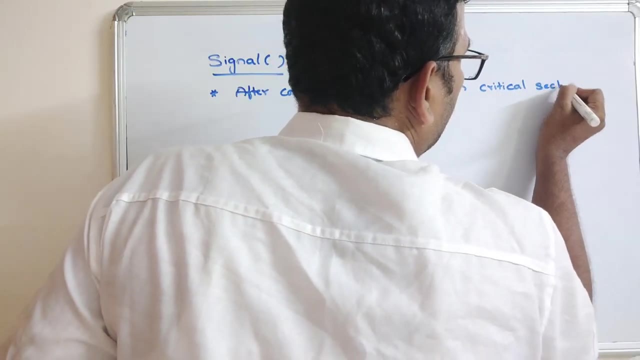 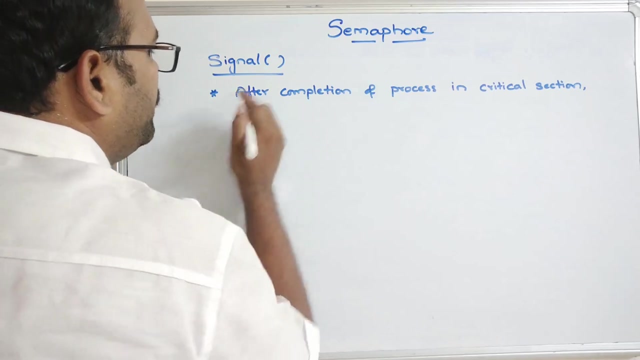 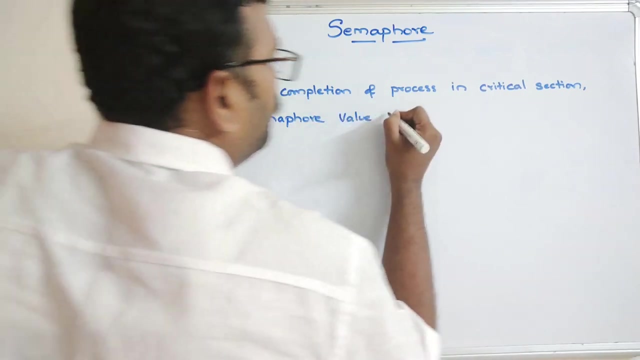 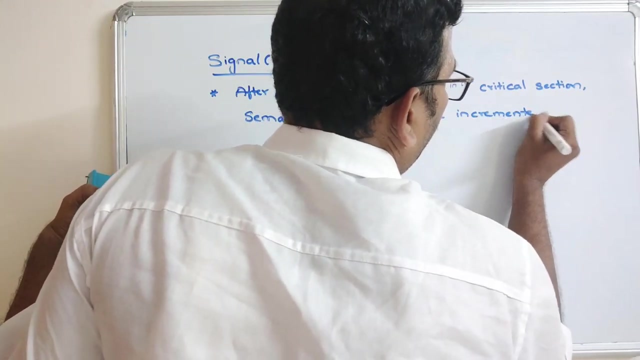 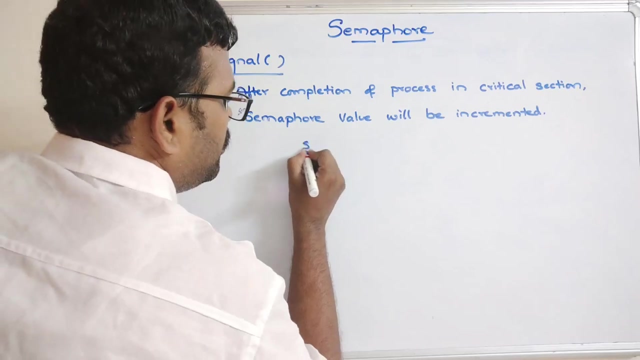 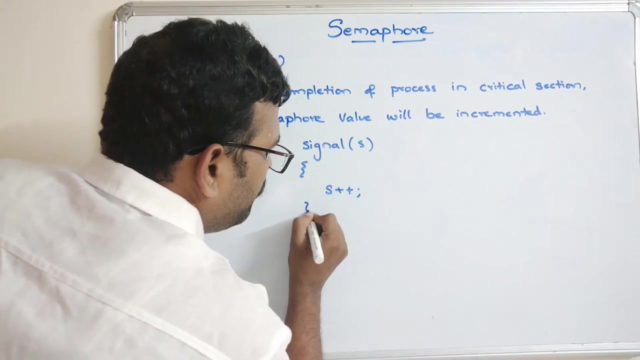 after completion of the process: in critical section: in critical section: immediately the semaphore value will be incremented. semaphore value will be incremented. value will be incremented So immediately. signal of yes. that is a semaphore: yes plus plus. immediately after completion of the process: execution: immediately the semaphore value. 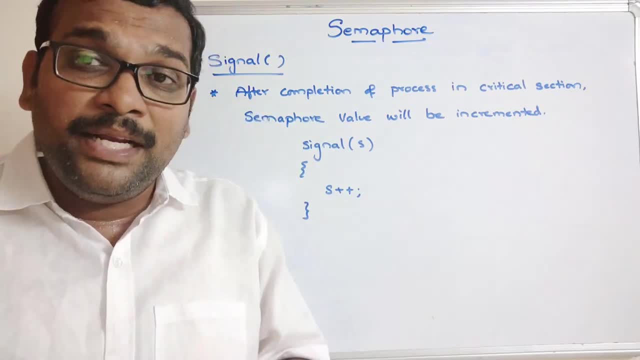 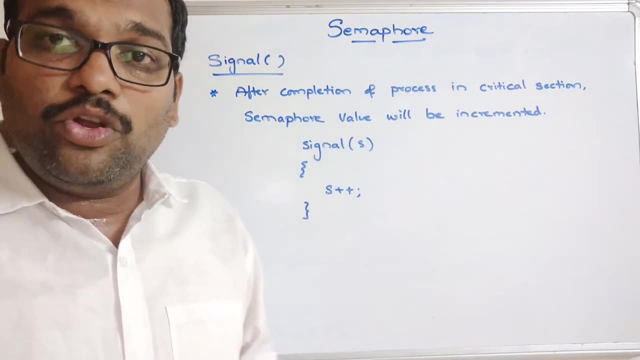 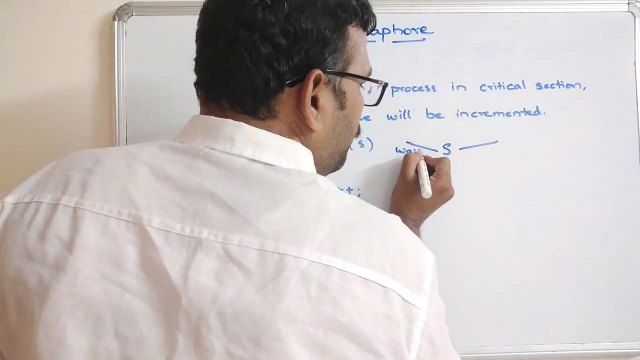 will be incremented, so it becomes greater than 0. that means some sort of resources are be allocated from the process and they are available for the other process. So immediately, yes is shared among different process. So in the wait signal we are using the S and in the signal 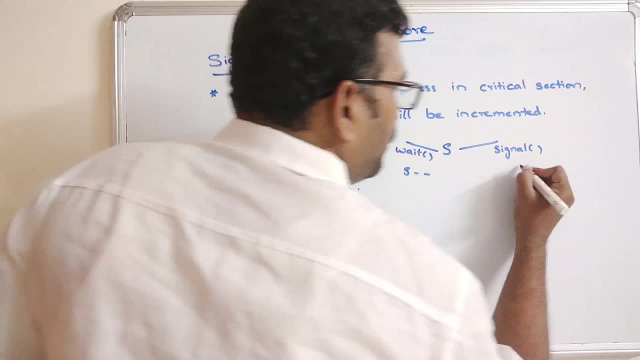 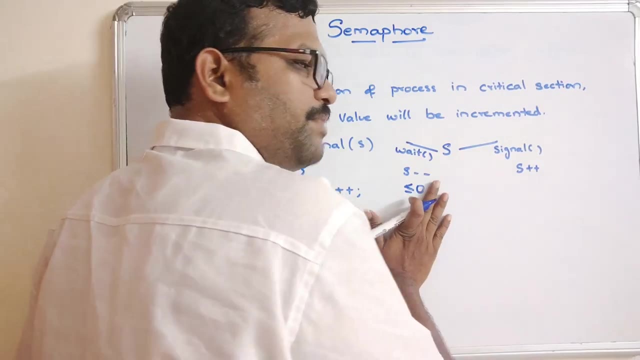 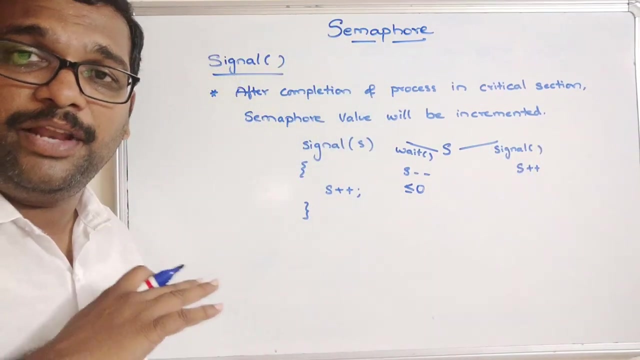 we are using the semaphore, Here we are using the decrement and here we are using the increment. So, whenever it is less than or equal to 0, it will wait until the resource is available, and here automatically Yes plus plus. once the process have been completed, its execution immediately S will. 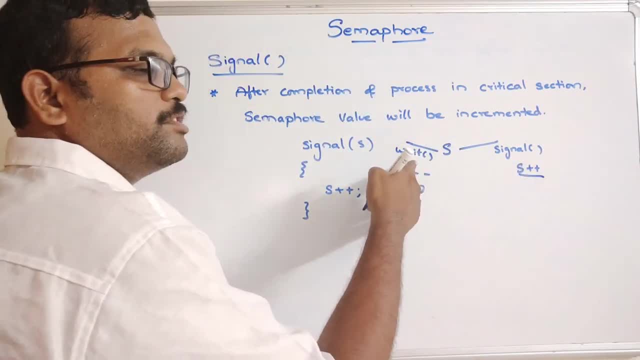 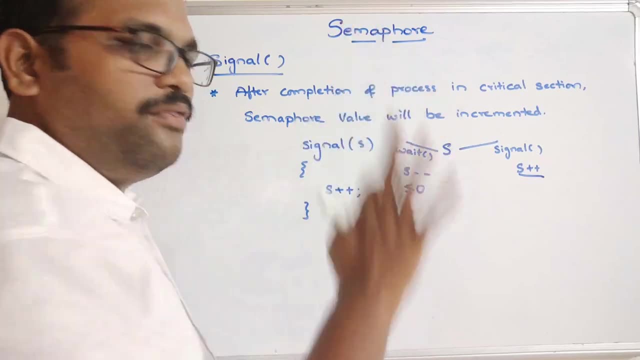 be incremented automatically. if S is incremented automatically, S will be greater than 0. if S is greater than 0, the resource is available, so some other process can avail the resource immediately. it will be allocated for another process and S will be decremented. So this: 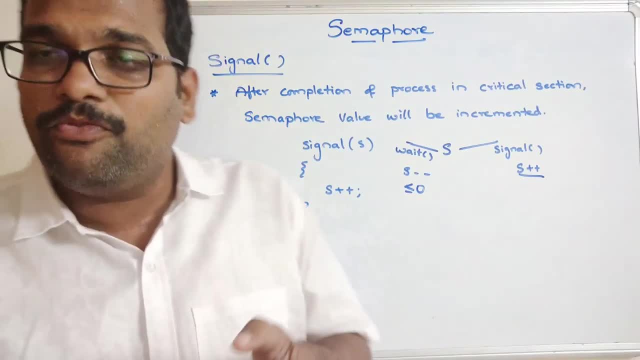 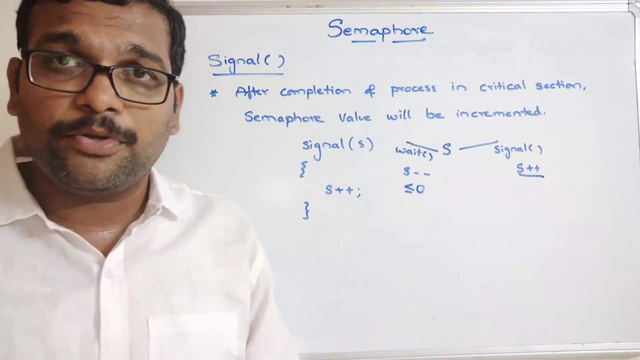 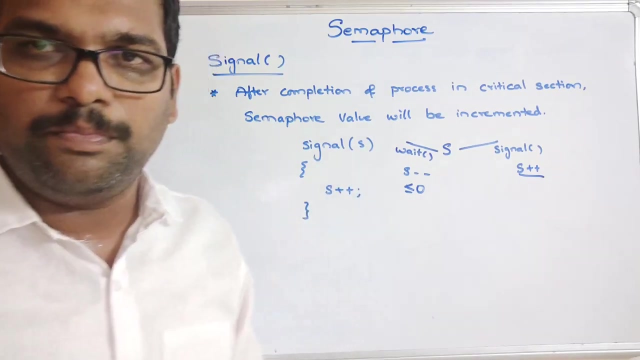 is how the critical section problem will be solved: with the help of wait and signal procedures, and both the procedures are the atomic procedures. That means after one, after completion, successful completion of one procedure, then only the second procedure should be executed, so no process should interrupt this one right. 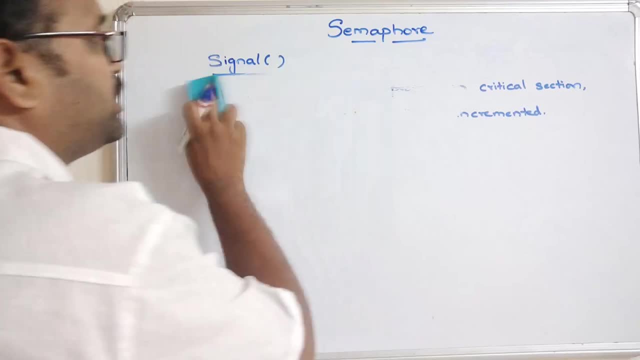 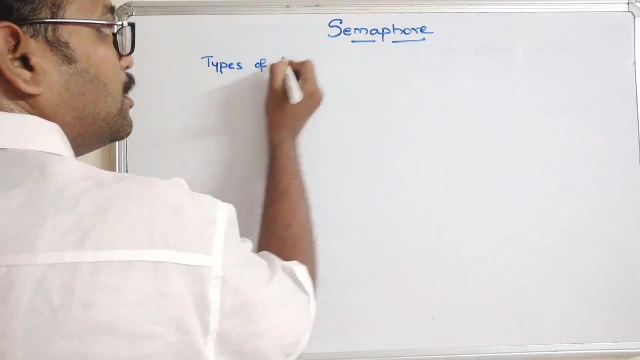 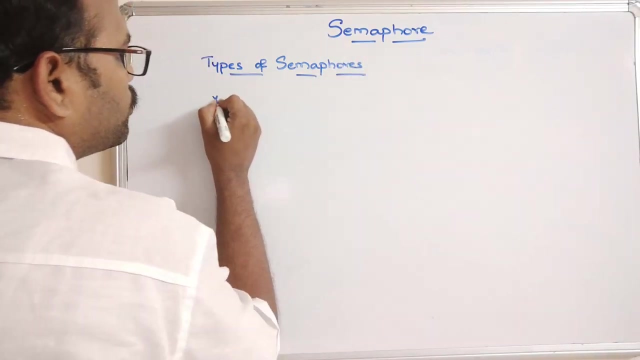 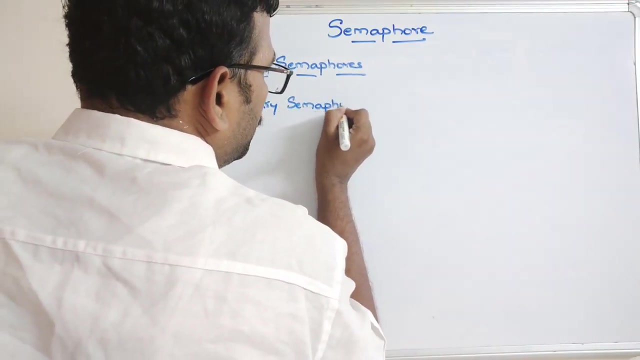 Now we will see the types of procedures. i mean types of semaphores. what are the different types of semaphores? Types of Semaphores: So there are mainly two types of semaphore, of semaphores. one is binary semaphore. binary semaphore so where the value will. 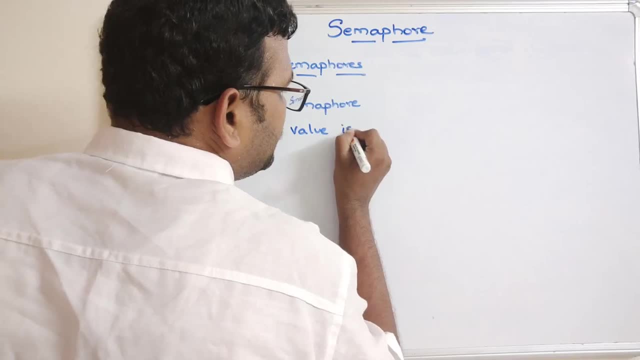 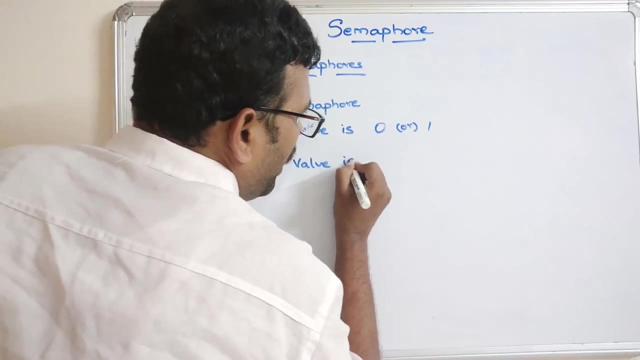 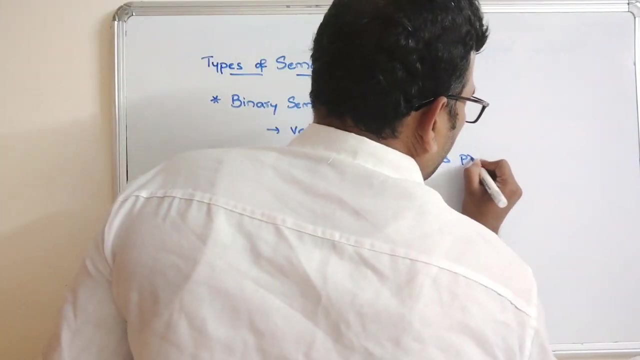 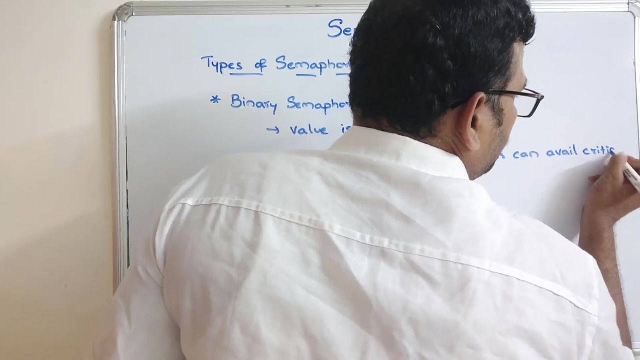 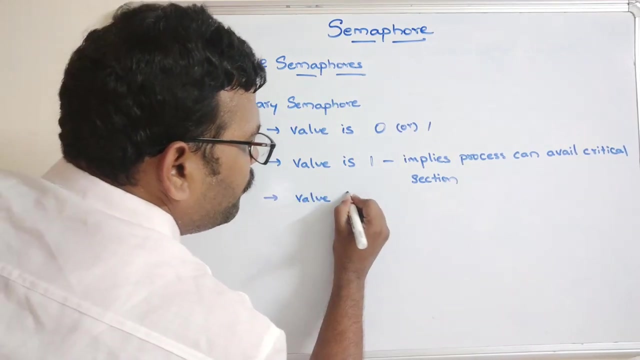 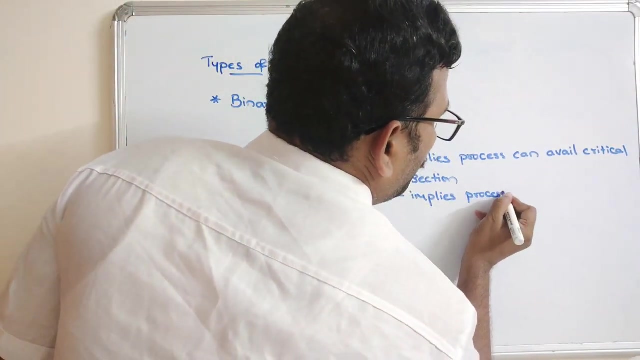 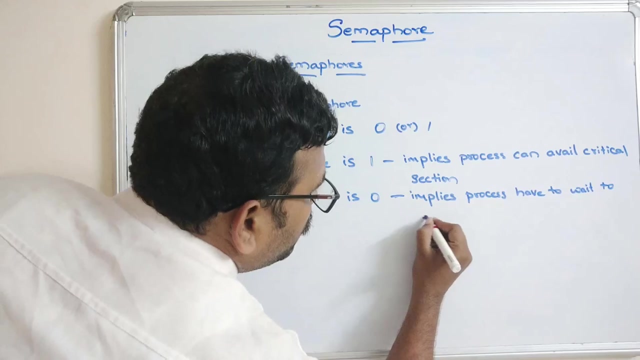 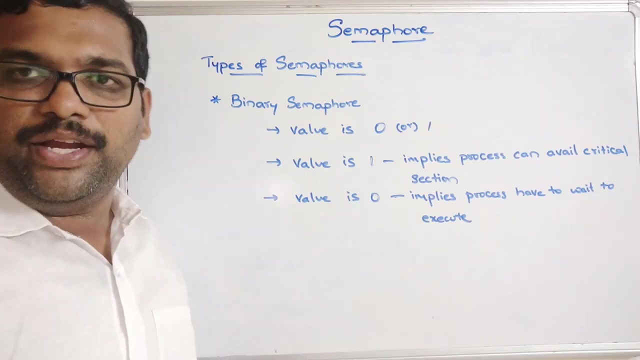 be where the value is either 0 or 1. and if value is 1, value is 1, implies implies process can away critical section, critical section. and if value is 0, if value is 0, implies process have to wait to execute. that means some other process is being executed, so it has to wait. and the second category: 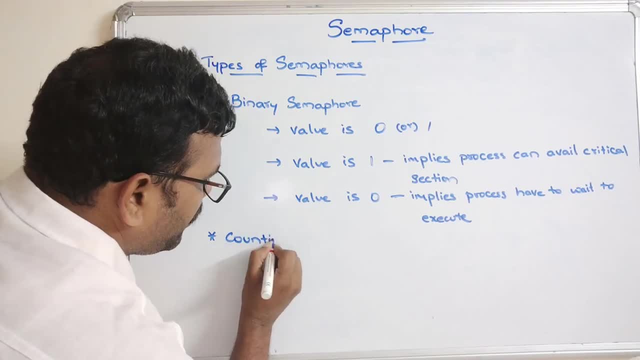 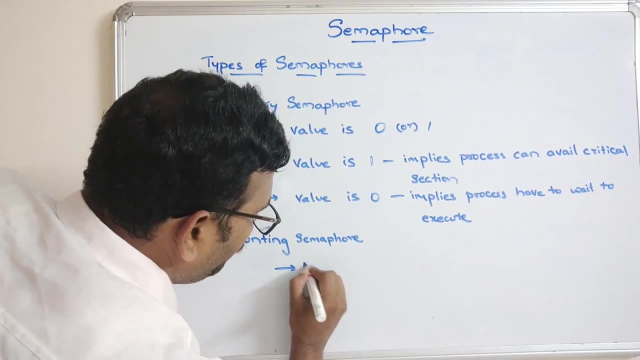 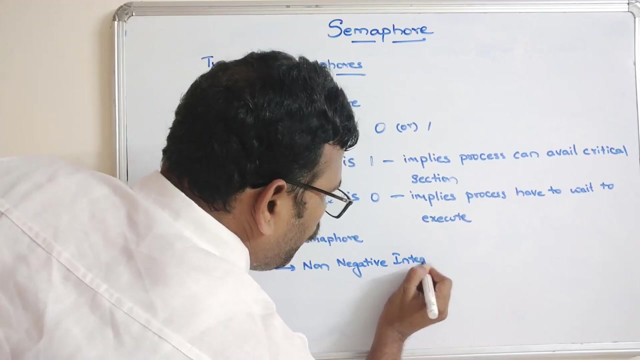 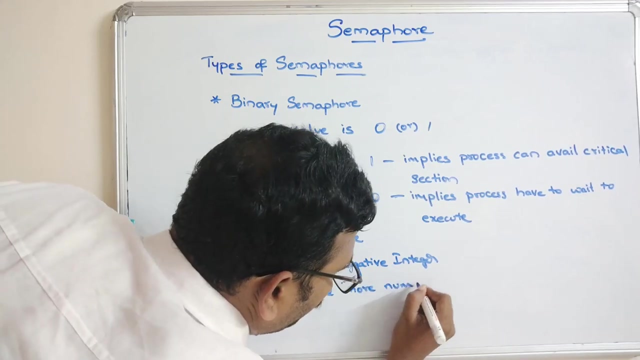 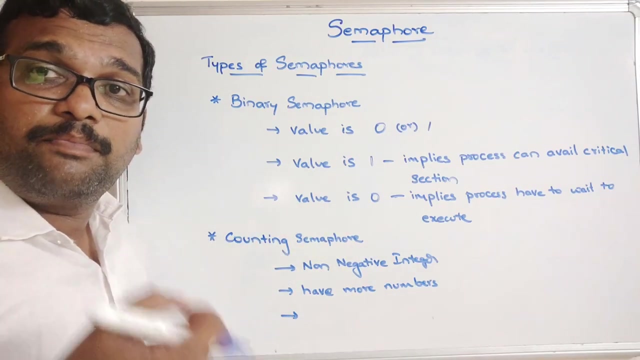 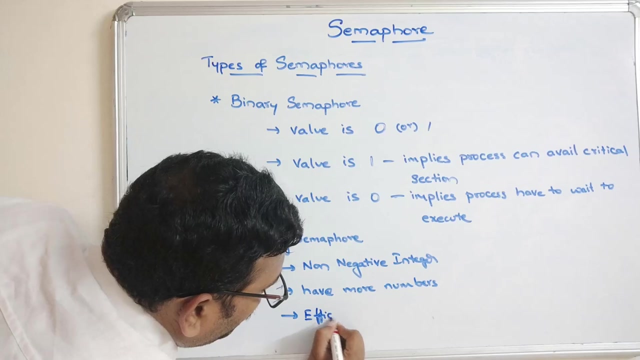 of semaphore is counting semaphore, counting semaphore. so here it will be a non negative value, non negative integer and will have more value, numbers, more numbers. and this type of semaphores are mainly used for using the pool of resources. there are multiple resources, right, so it is used for. 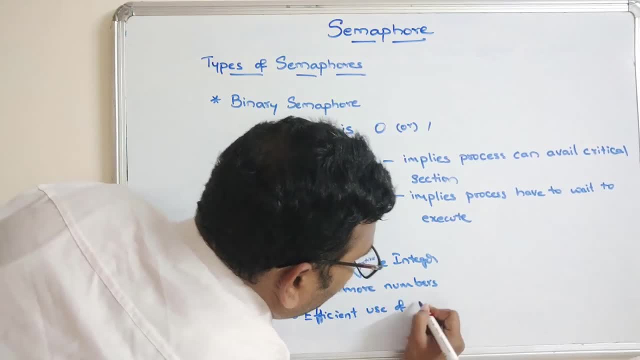 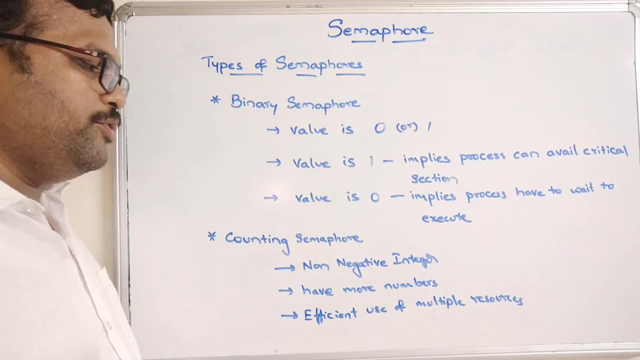 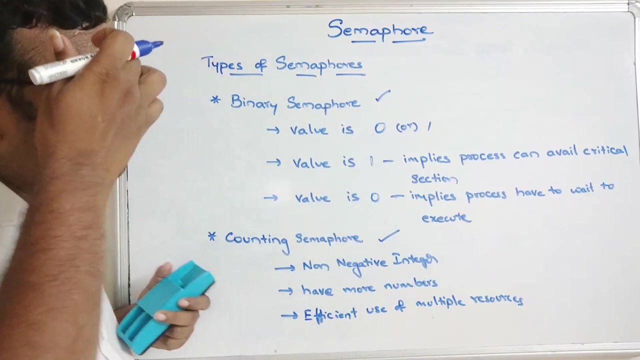 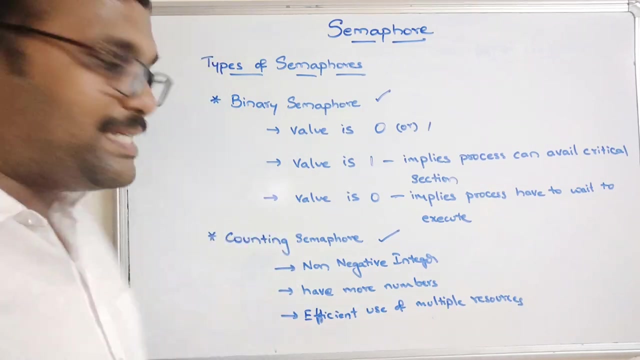 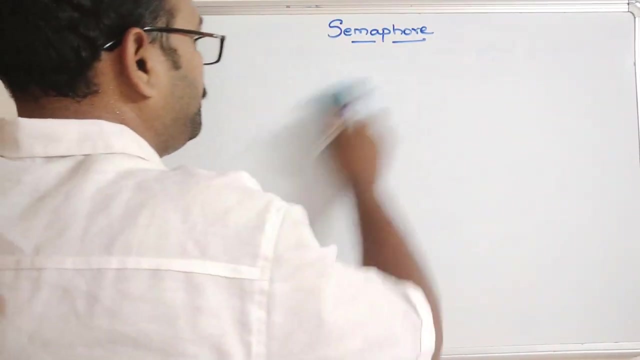 efficient use of multiple resources. if there are more than one resource, then we can use this counting semaphore. so these two are a different types of semaphores: binary semaphore as well as the counting semaphore. so hope you understood this one. so let's see the advantages of semaphore. advantages of semaphore. so 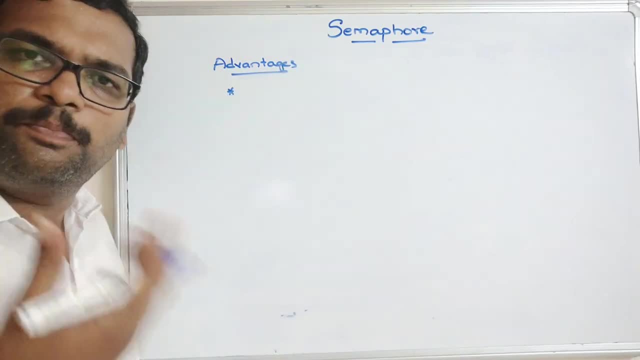 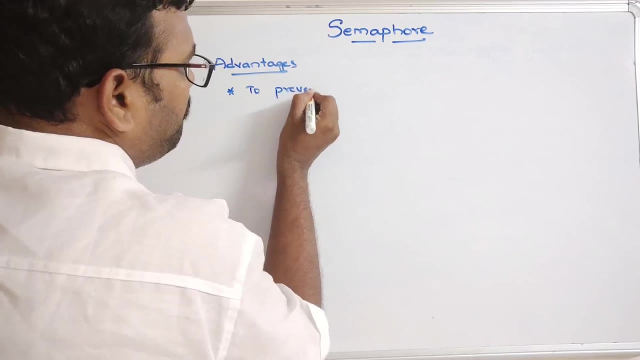 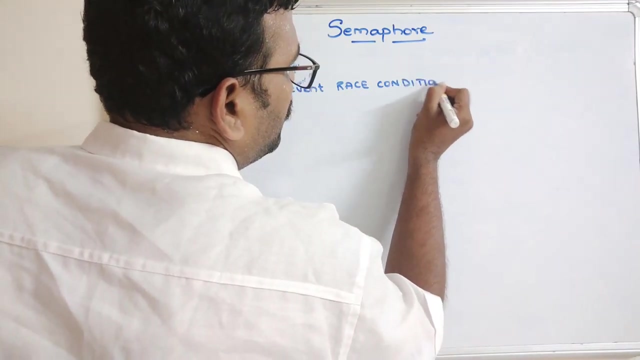 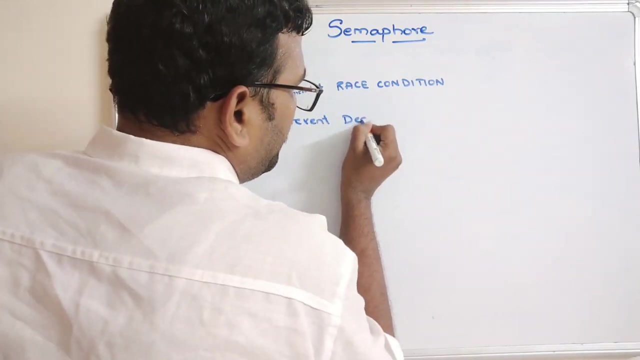 first advantage. we have discussed it just now. we are using the semaphore to prevent the race condition in order to prevent the race condition. so so, to prevent race condition. and the second one, to prevent the deadlocks. to prevent deadlocks, that means if one resource is allocated to one. 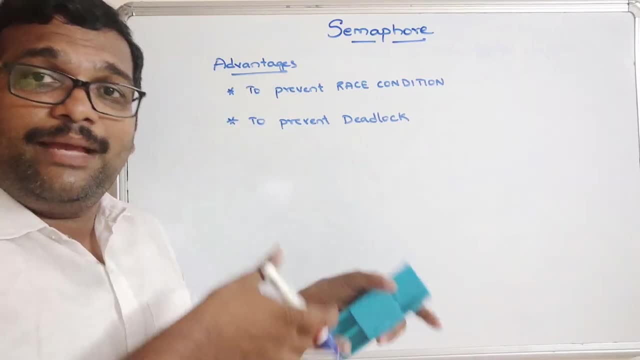 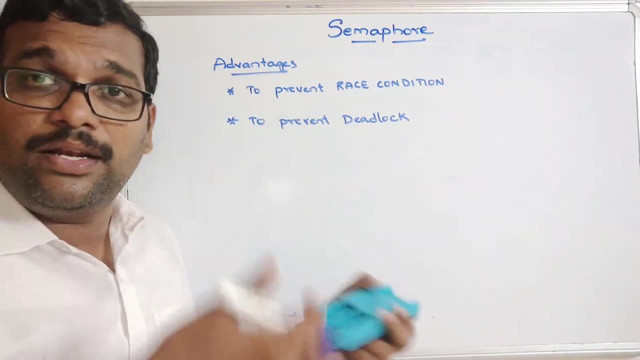 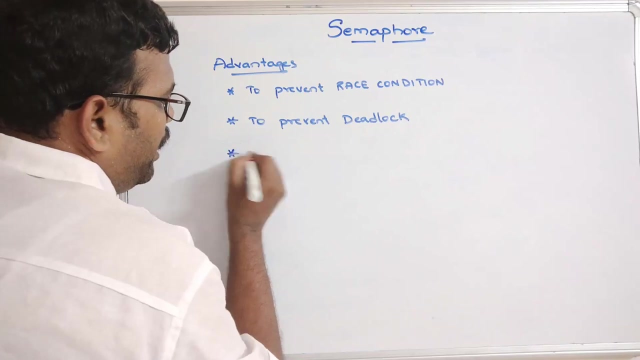 process and process is also waiting for the same resource, so that's a never ending process. that we call it is a deadlock, so in our further sessions we will discuss about the deadlocks, right? so in order to prevent the deadlocks also, we use this semaphore and to implement mutual 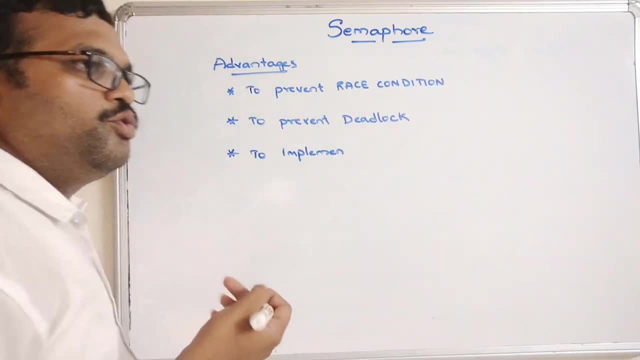 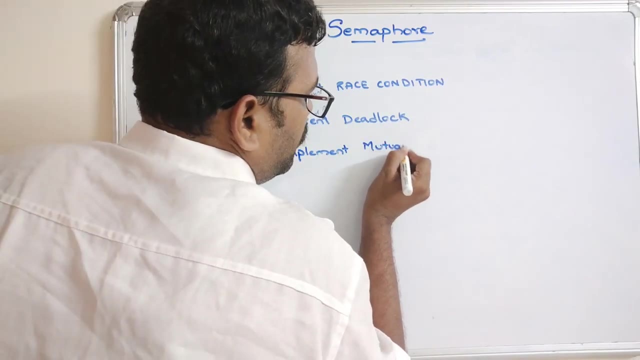 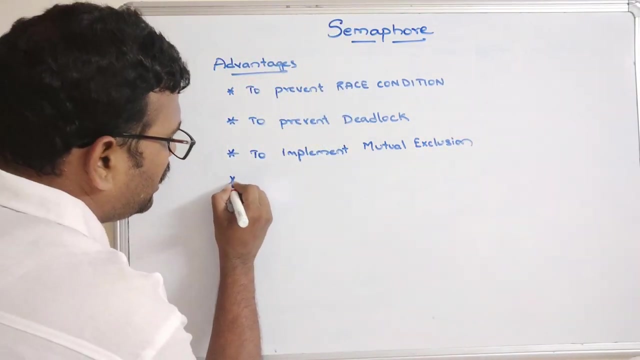 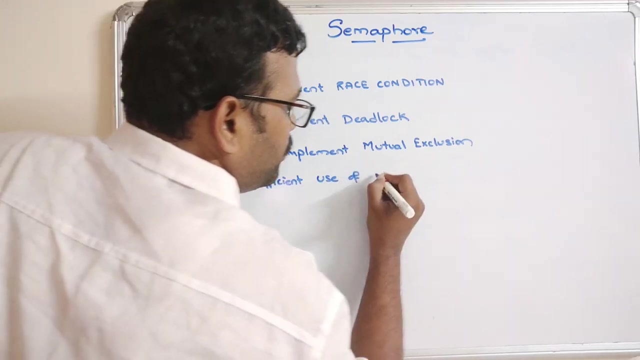 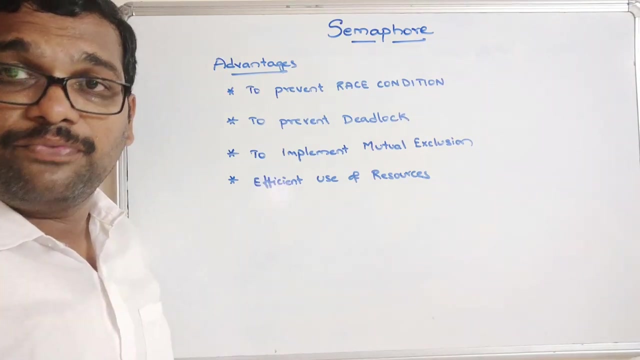 exclusion, which is a one condition, need to be satisfied for critical section problem. so to implement mutual exclusion, mutual exclusion and another one: efficient use of resources. just now we have discussed efficient use of resources. for all these reasons, we are going with the semaphore, which is a integer value. it is an integer value. now, what are the disadvantages? 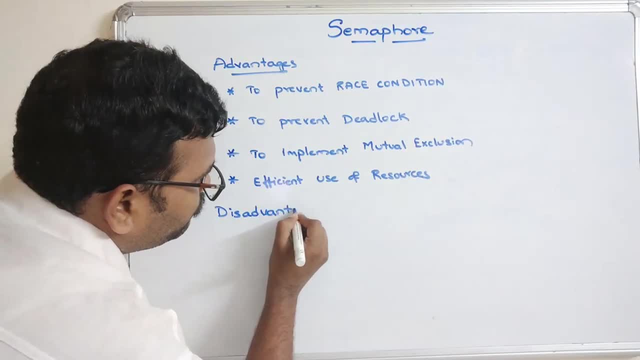 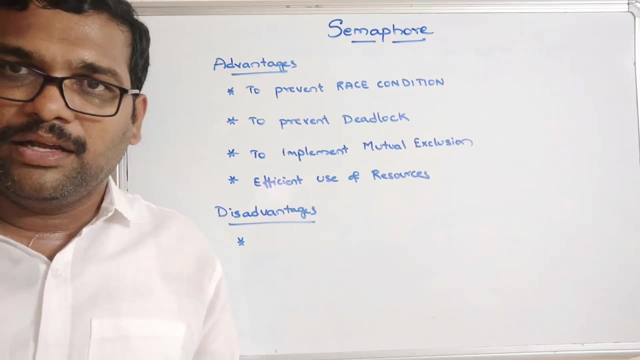 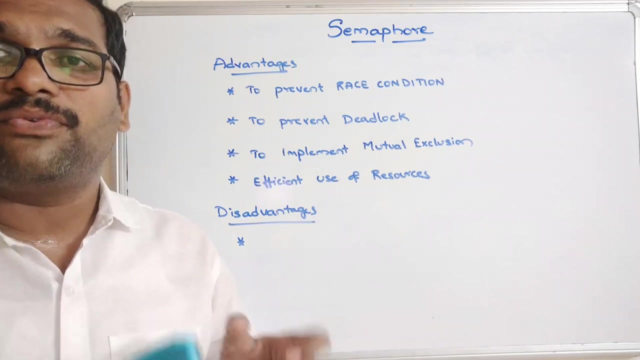 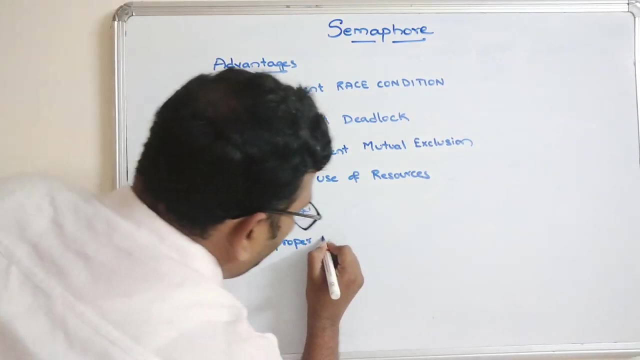 of semaphore. so obviously some sort of disadvantages will be there. so the first main disadvantage is we need to use this semaphore perfectly. so if you are unable to use this semaphore perfectly, automatically there might be a chance of getting a deadlock situation. so improper usage. improper usage of semaphore, of semaphore. 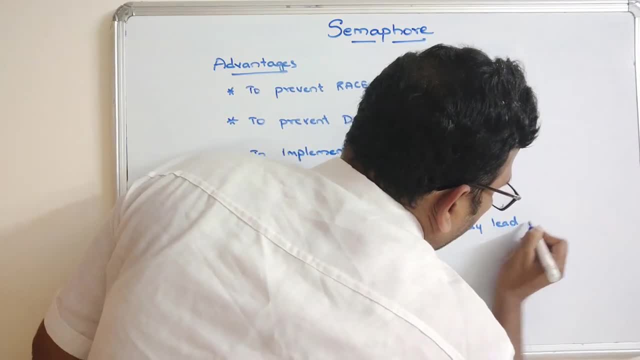 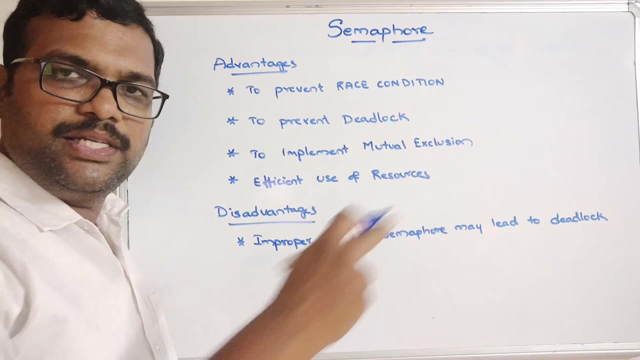 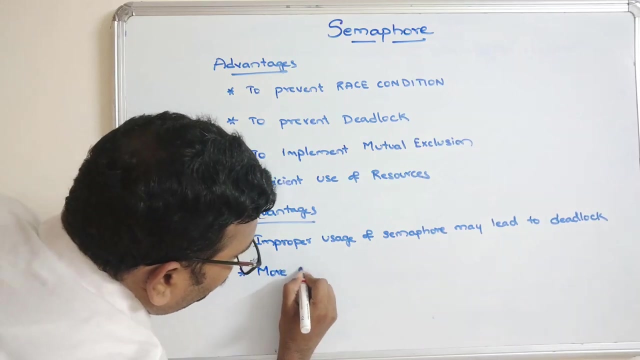 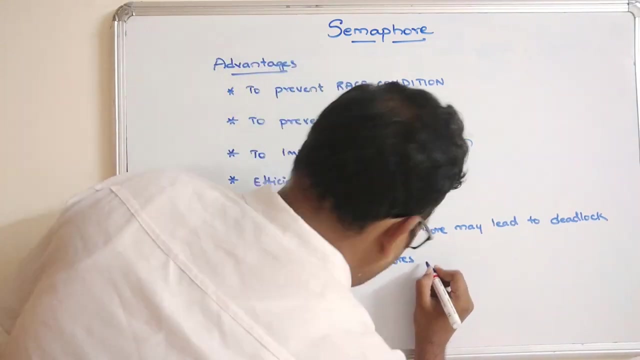 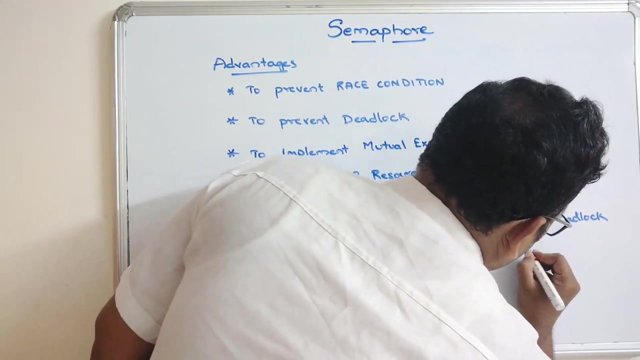 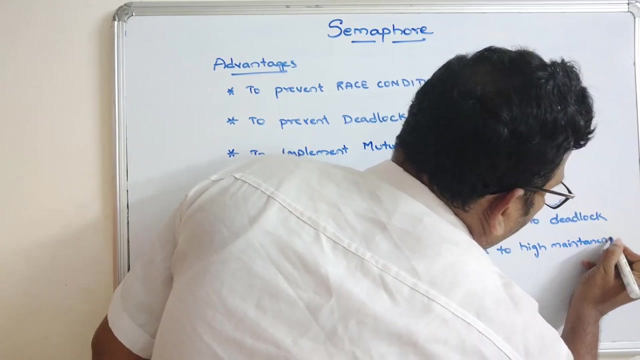 may lead to. may lead to deadlock situation, deadlock situation. in our further sessions we will see about the deadlock. what is what exactly the deadlock? and also more number of semaphores. if you are using more number of semaphores, force may lead to high maintenance and confusion. high maintenance and confusion- right more.